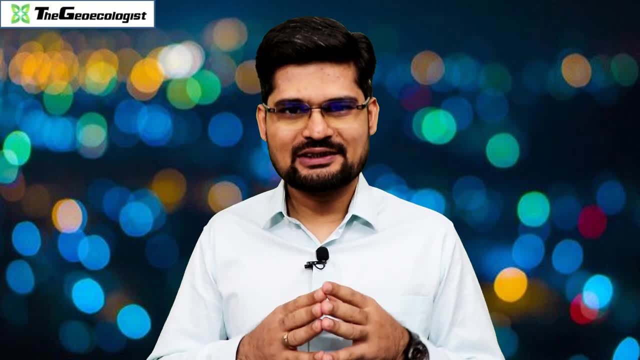 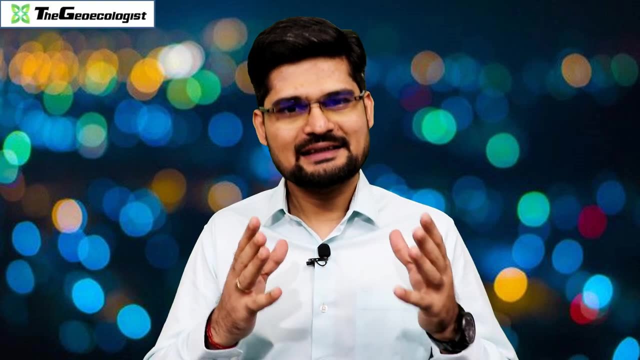 Hello everyone, welcome to the Geoecologist. I am Dr Krishnanand and you have been watching my videos on various topics of geography, environment and research methodology on my channel, the Geoecologist. So if you are new to this channel, consider subscribing our channel. 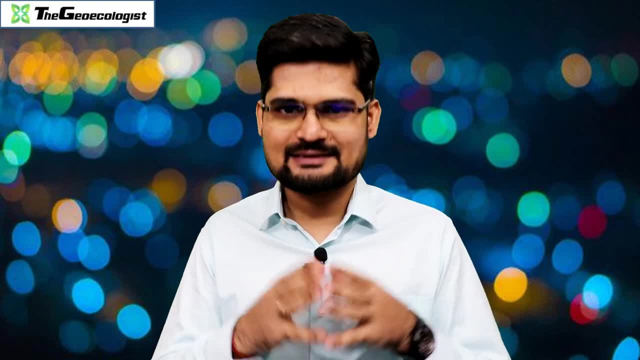 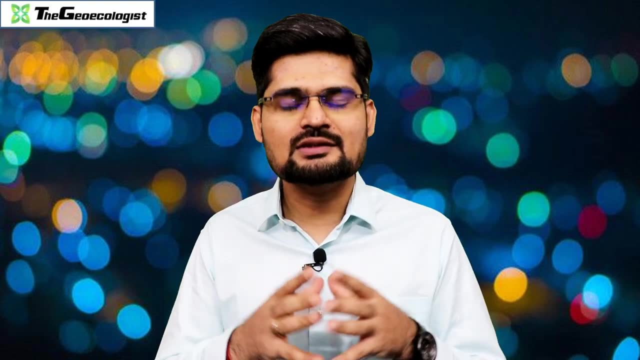 and also for the earlier videos. you can go to the playlist section Now. in today's session on world regional geography, we are going to talk about the North American region or the North American realm, So the details of this North American realm in terms of mainlands, islands. 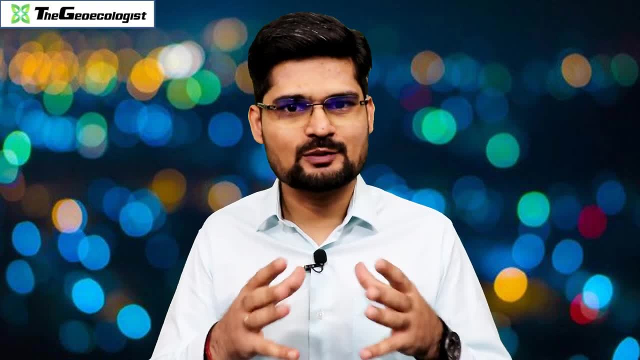 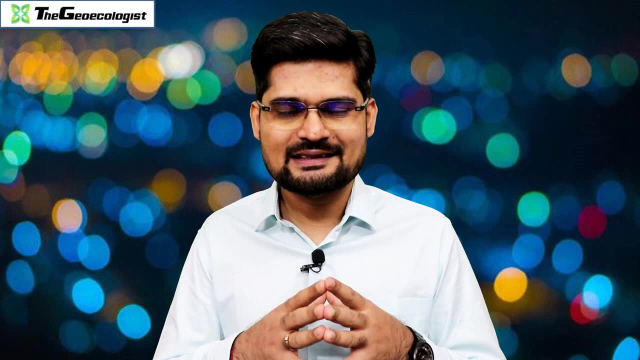 gulfs, seas and several other physiographic units alongside the human geography would be discussed in today's session. So watch the video till the end to learn about the North American realm in details. and also, before we go ahead, don't forget to subscribe to our channel and 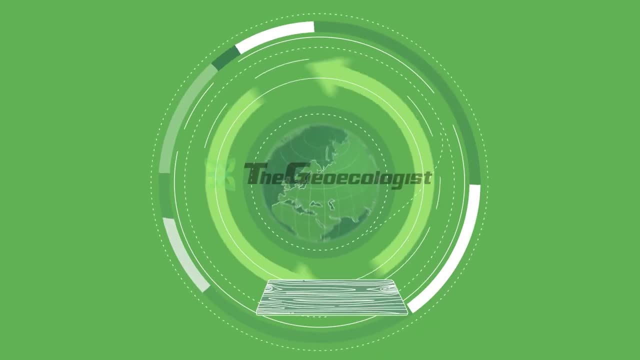 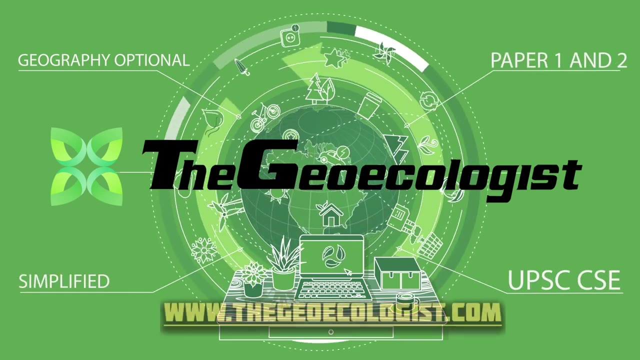 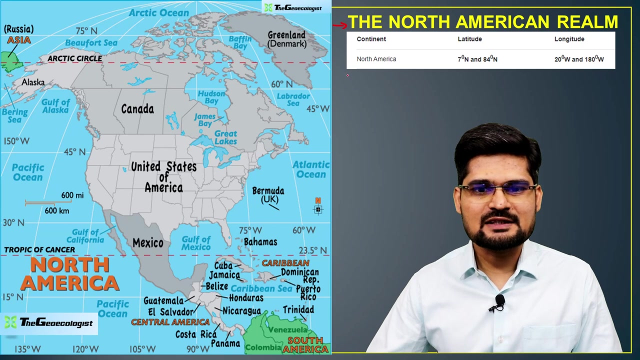 do share the videos with others as well. So now let's discuss about this North American realm. So if you observe, the first important thing here is the location of this North American region. So this is 7 degree north, 84 degree north latitude and 20 degree west to 180 degree west longitude. So if you demarcate it carefully, 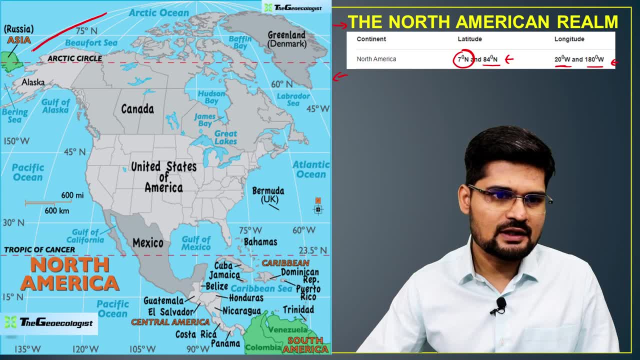 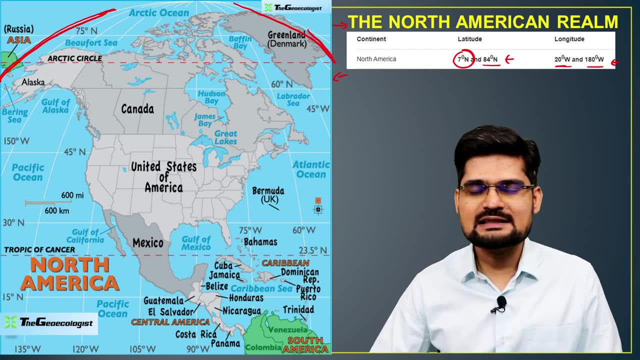 it falls somewhere about this particular location that is 180 degree here and this particular location that is about 20 degree here. So this is the longitudinal extent and then if you observe the latitudinal extent, so in latitudes, 7 degrees here somewhere, and above this 7 degree, till what? 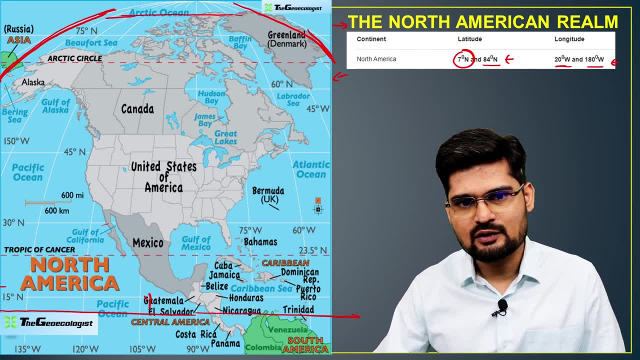 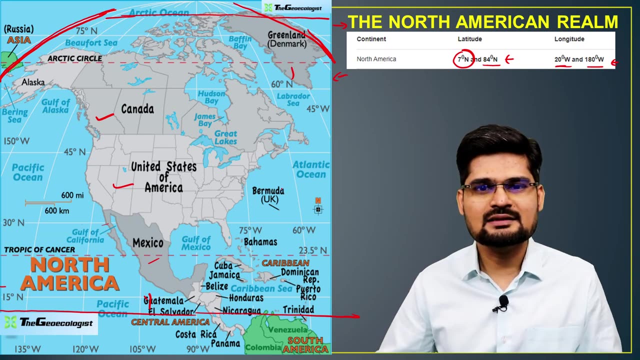 you observe is 84 degrees. So this is somewhere 84 degrees close to the poles. So this is where this particular North American realm lies and this is majorly dominated by few countries. So you know Canada, United States of America, Mexico and several islands like Greenland and others. So this is what 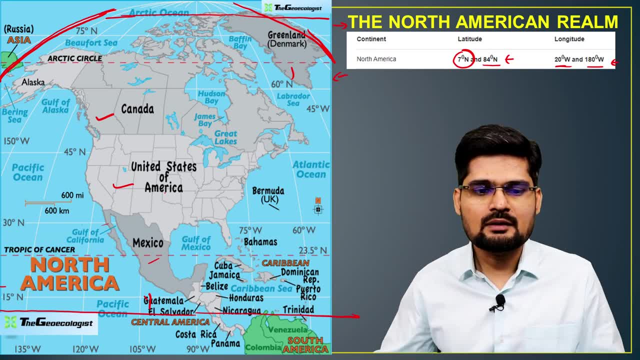 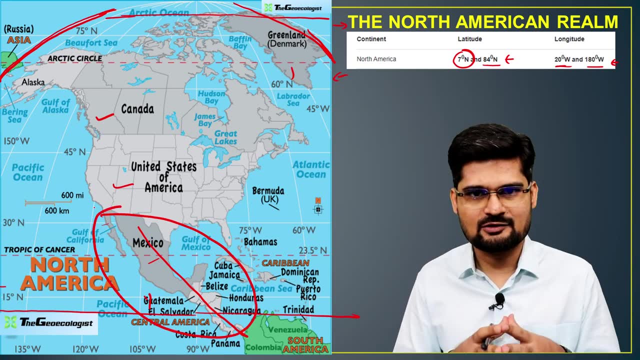 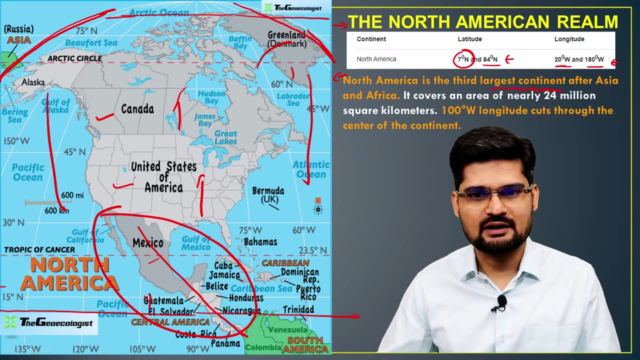 we are going to learn about in North American realm and remember Mexico and the other subsequent. this particular will be learning in this separate lecture in Middle American realm. Now, if you observe carefully that North America, if you observe, is the third largest continent after Asia and Africa, 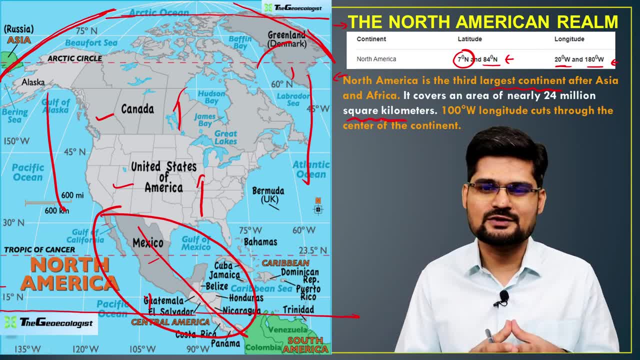 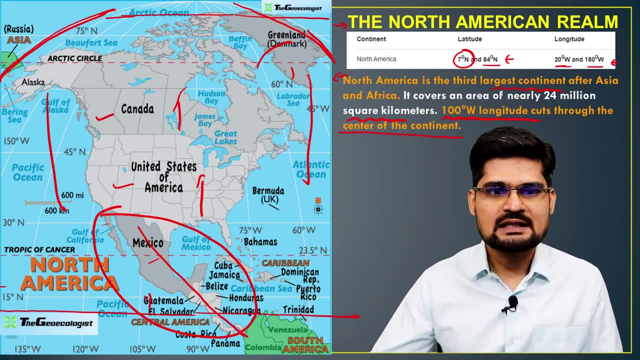 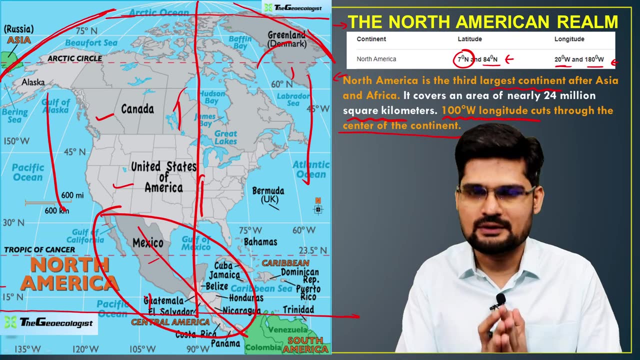 and it covers nearly 24 million square kilometers of the world and remember, 100 degree west longitude cuts through center of the continents. So almost this particular longitude, if you observe, cuts through the center of continent. these are the basic data or information which are important. 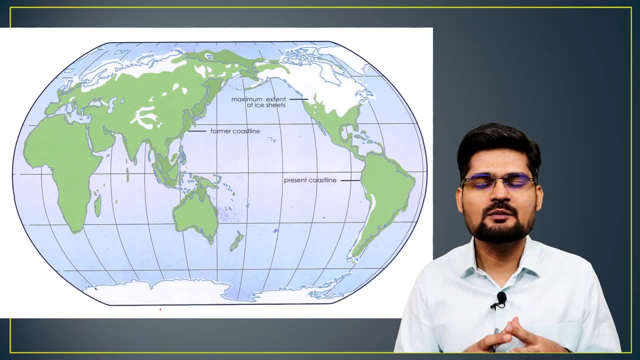 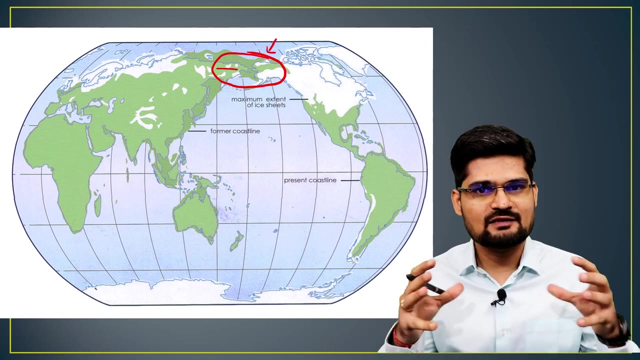 Now, if you observe further that this particular realm was connected with Asia once upon a time, this connection was there, and why we are talking about it? because it's very important in geography to understand that once these lands were connected and after the ice melted in the Pleistocene glaciation, they were together and once the melting happened then they got branched away. 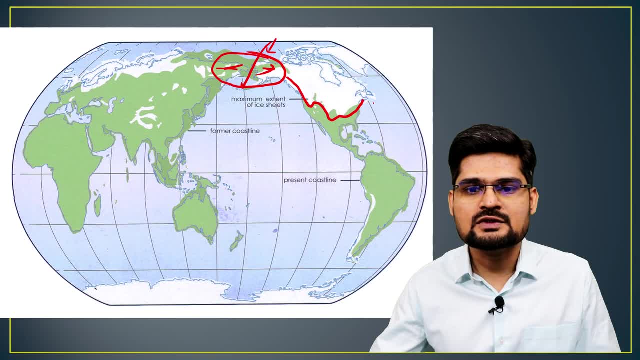 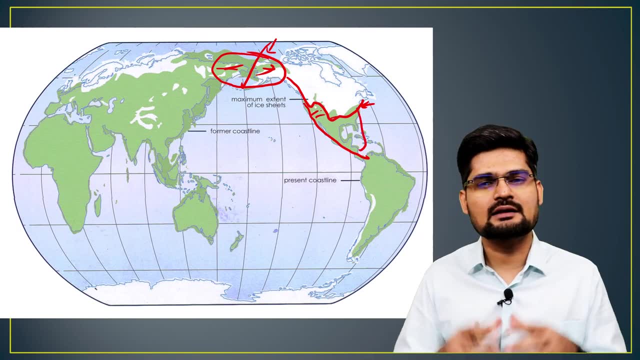 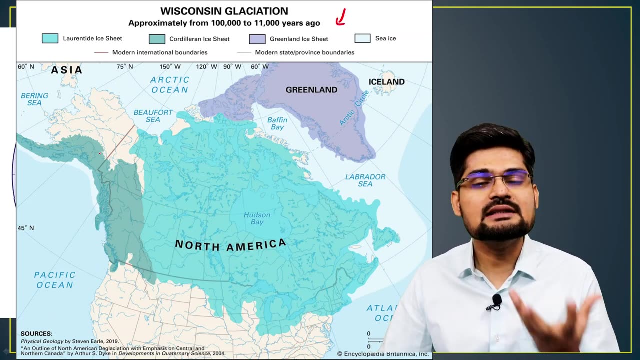 and during Pleistocene the glaciation happened Until almost the southern part of Americas as well. So if you observe this particular Middle Americas, so almost north of Middle America, till that point glaciation had an impact. So we can observe in this particular glaciation impact and see that how glaciated landforms were created at the end. 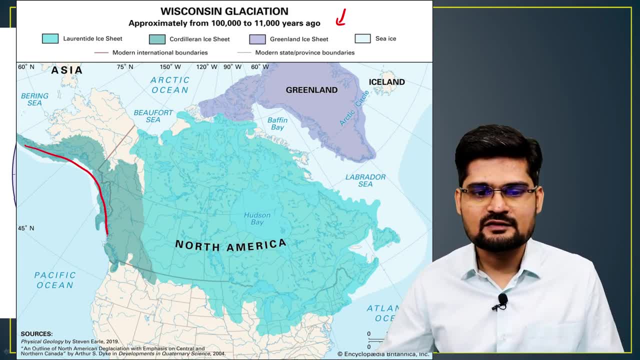 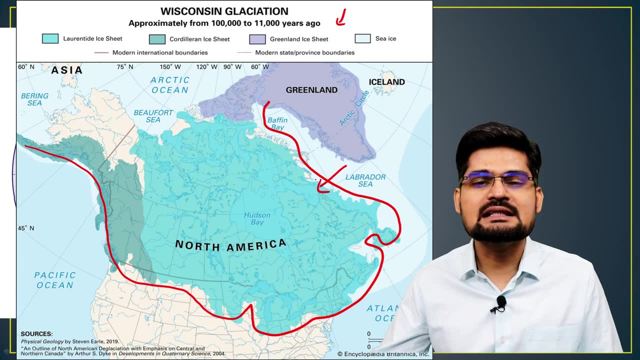 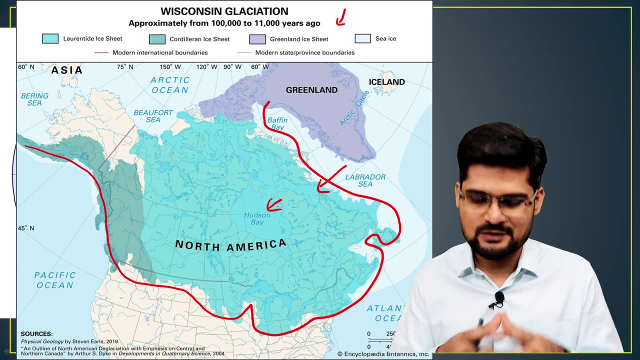 of Pleistocene. So, if you observe, these are the areas of North America till which the glaciers had an impact and what happened because of this. These areas have numerous lakes, bay areas and several other fragmented landscapes because of the glaciation in the earlier times. So let's look into 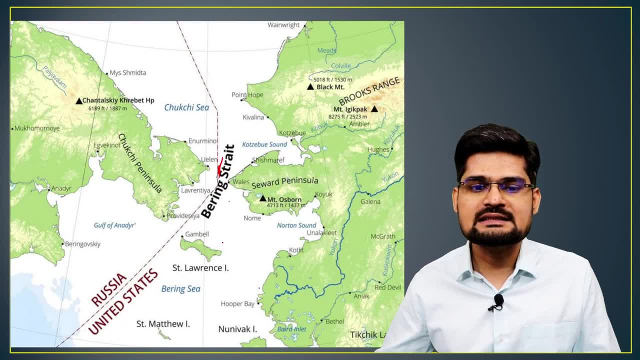 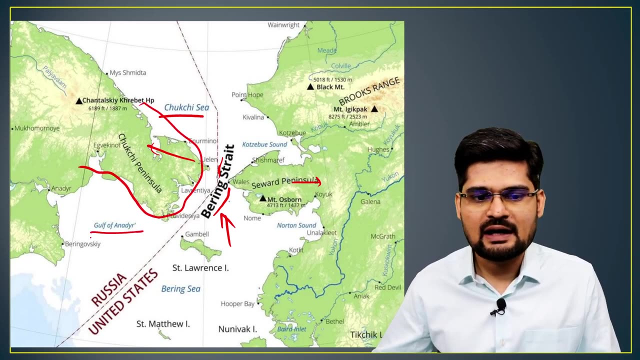 this that this particular strait was formed once the sea level rise started to happen and the continents of Asia and North America got separated by Bering Strait. So areas around Bering Strait, if you observe, this is Tukshi Sea and this is Tukshi Peninsula. if you observe Gulf of Anadir, then you 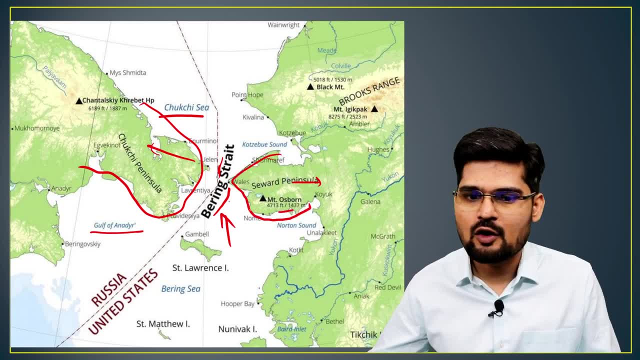 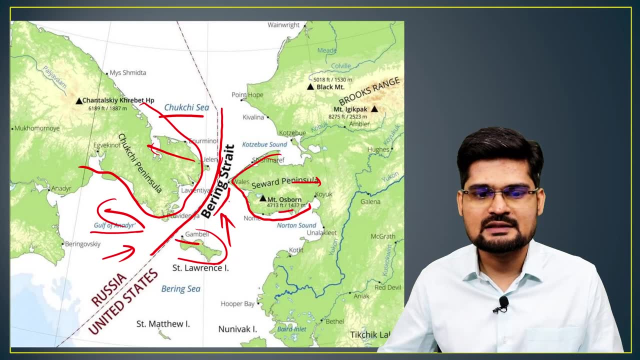 have this particular seaboard peninsula here right, Mount Osborne, very famous, and this is where the Bering Strait lies. Here is the St Lawrence Island. So this is Russia and this is United States, if you observe carefully. Now let's look into the physiography of the North America. 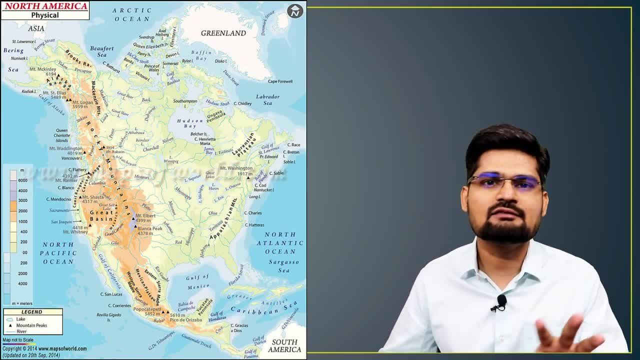 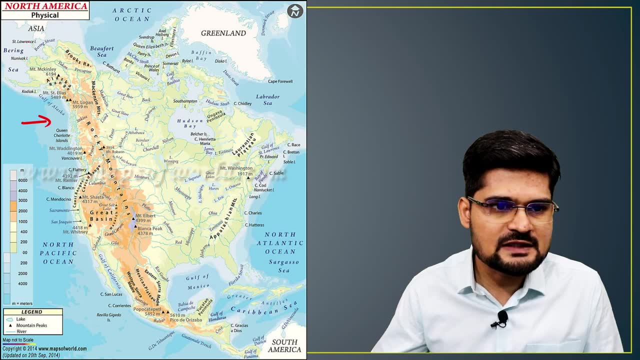 and let's look into the coastwise physiography first and then we'll look into the mainland. So if you observe on the western coast of North America first, so right from this particular Bering Strait we come down onwards, this is Bering Sea area, then particular area, if you observe here: 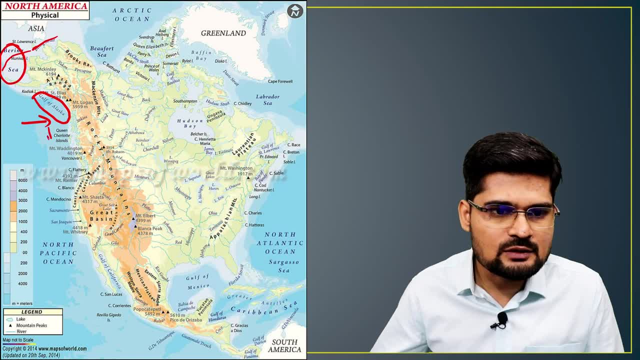 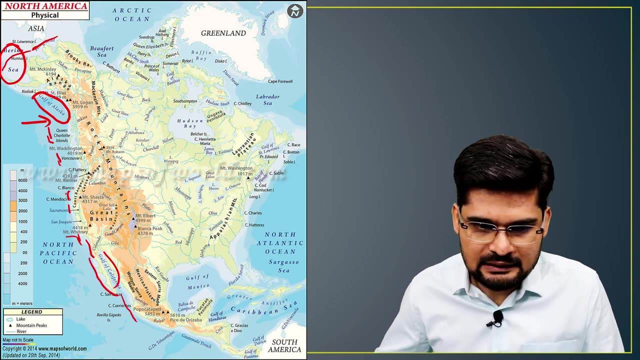 is Gulf of Alaska Here. then as you go down south, going to the Queen, Charlotte Island and Vancouver, then further, if you observe these coastal ranges are there, then you have Mount Whitney. here here is your Colorado and Gulf of California out here. then, as you go down south, then further you have the Mexican. 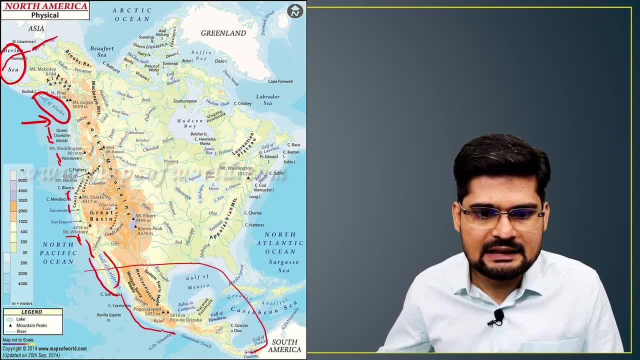 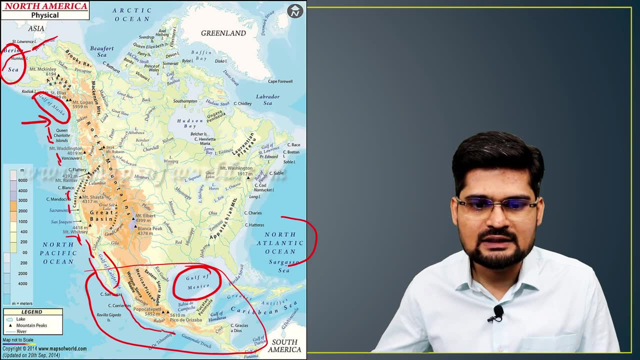 Plateau and its nearby areas, and this area will cover in details again in Middle American realm. Now, if you go, go here, here is Gulf of Mexico on this particular side, and this is North Atlantic Ocean. this is Pacific Ocean, As we know. now let's look into the northern portion here, where Arctic Ocean is there and you have 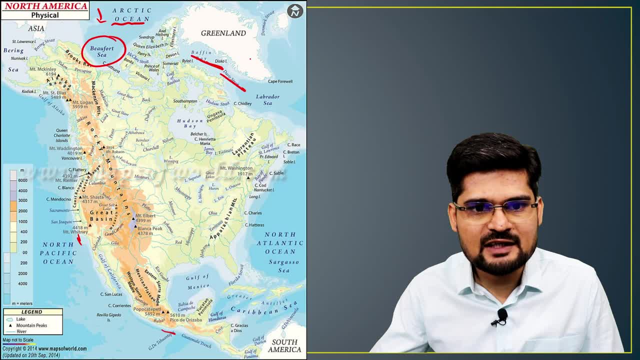 Buford Sea, then you have Baffin Bay- here there is straight between Greenland and Canada right, Gulf of Boothia, then you have Hudson Strait, then you have Laurentian Plateau here and Hudson Bay here right. then you have Gulf of St Lawrence here, Bay of Fundy here, then you have, furthermore, if you come here, 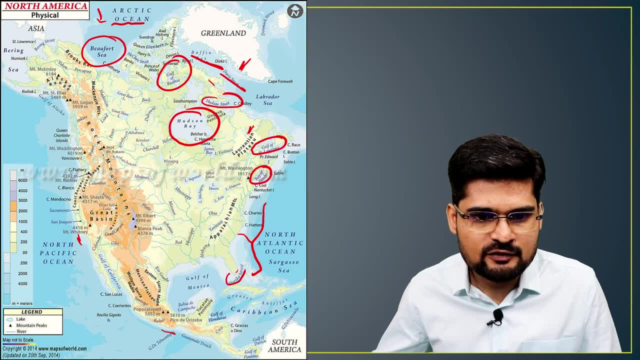 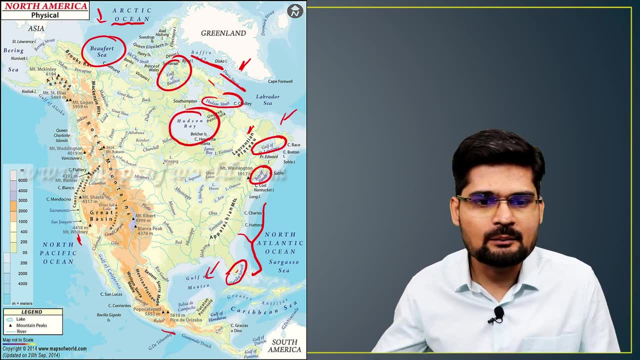 you see that there is a continental shelf in this portion. you have Florida Strait and Gulf of Mexico. So these are the coastal features, If you observe, of North America. This is North American continent. further inside, if you go, there are many other physical features which we are going to look. 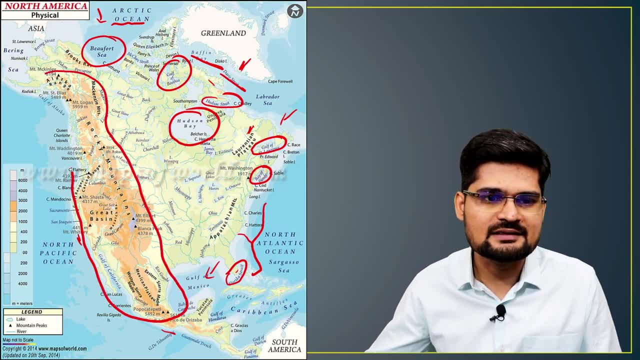 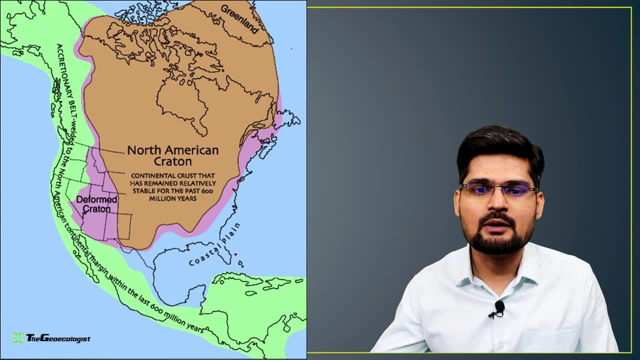 So can you see a prominence of this Western Cordilleras here, and why is it called Western Cordilleras? because it's like a cord, cord of several chains of mountains. So let's understand further about a little of geology of this North America. 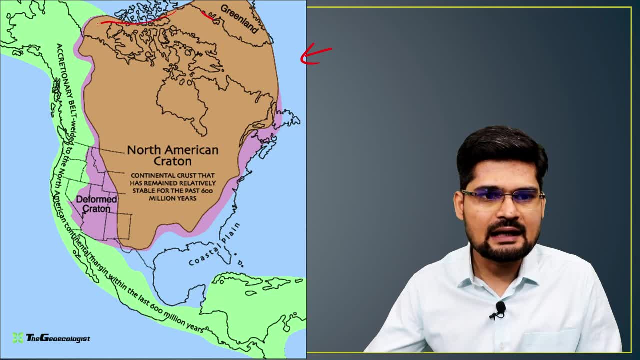 So if you look into the geology of North America, the Greenland and this particular portion, if you observe, is the North American Craton, the Cratonization process, and here it has not moved or there has not been much of movement or dynamicity since 600 million years. so this 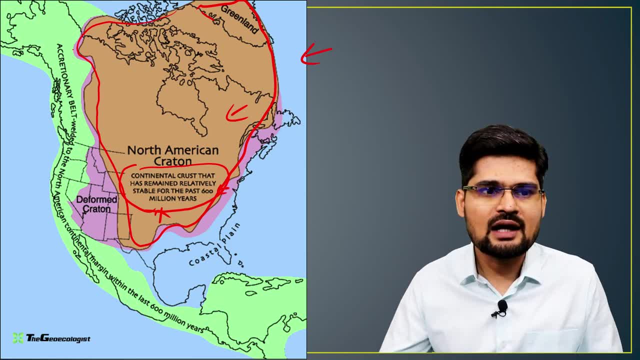 is supposed to be the oldest block of North America, and then you have an accretion zone alongside the coastal area of Pacific. here this is the accretionary belt. We are a lot of coastal belt, mountains are there in accretion and these are also almost. 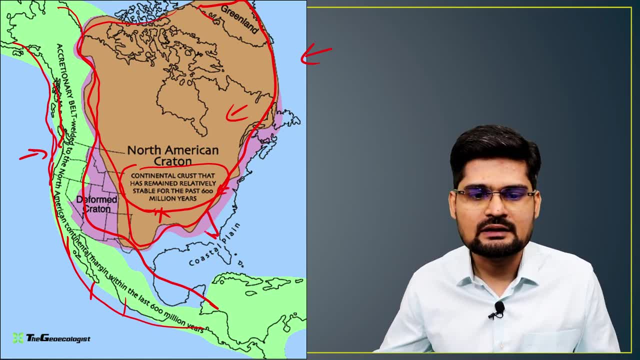 540 million years old. and here is the coastal plain on the other side right. So this is basic geological structure and if you observe on the basis of this geological structure, And here is the coastal plane on the other side. So this is basic geological structure And if you observe on the basis of this geological structure, 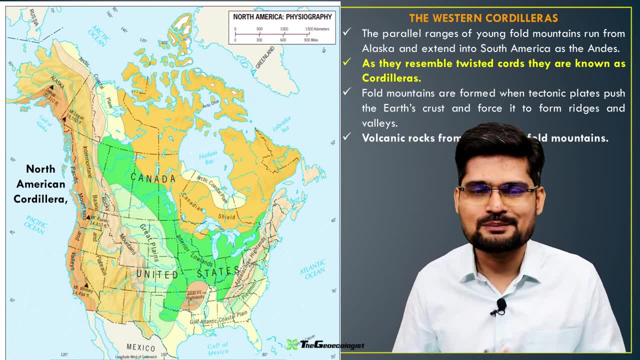 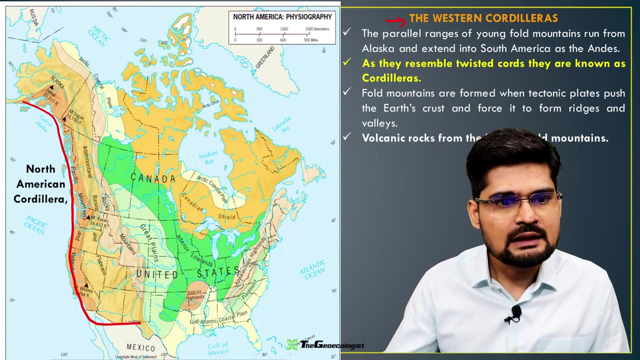 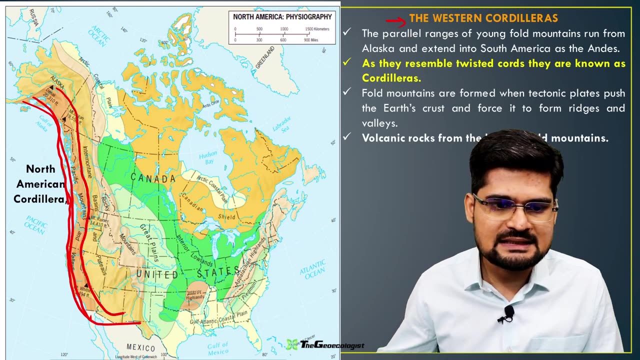 the geomorphology of north america, or we say, physiography in simple language. so here is the western cordillera, this entire location here, if you observe, and what you observe here, the coastal areas are pacific mountains right and then you have the intermountain basin. here is the basin. 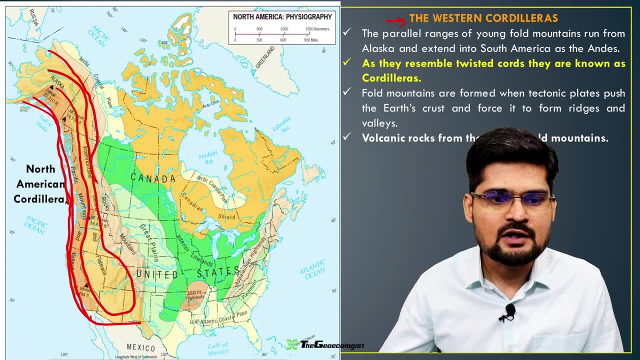 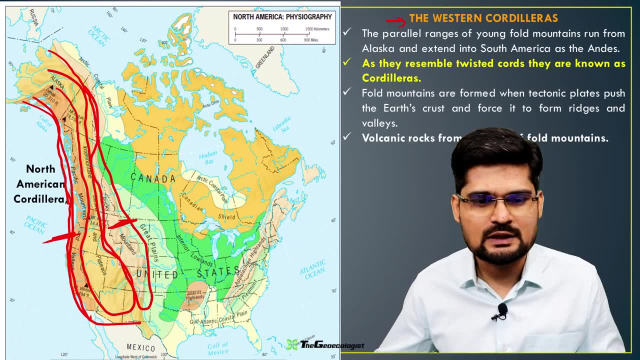 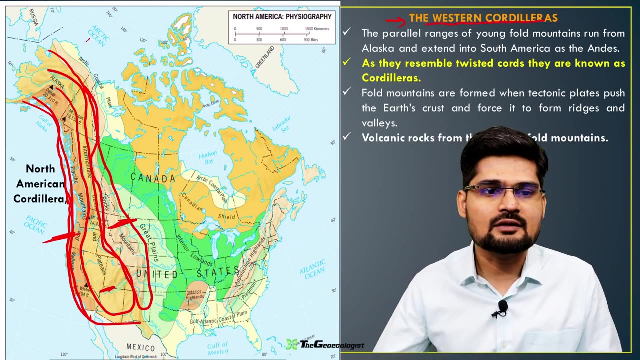 structure in between, and then you have the long chain of rocky mountains here. so between rocky mountains on one side and the coastal on one side, or pacific rim on one side, what you have is the intermountain plateaus and basin structure. so this is where western cordillera is, here on the 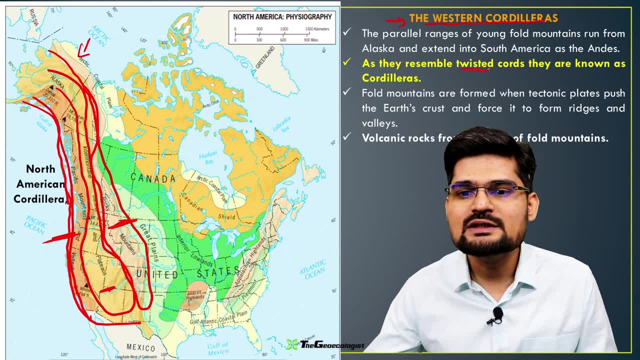 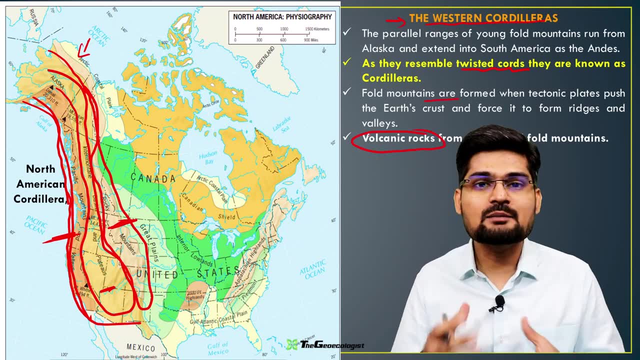 western part. now, what is important here? they resemble twisted cords and they are called cordilleras, as we know, and they are full mountains and they have a volcanic base structure. so, volcanic base structure because of the subduction zones and as we have learned in the process of 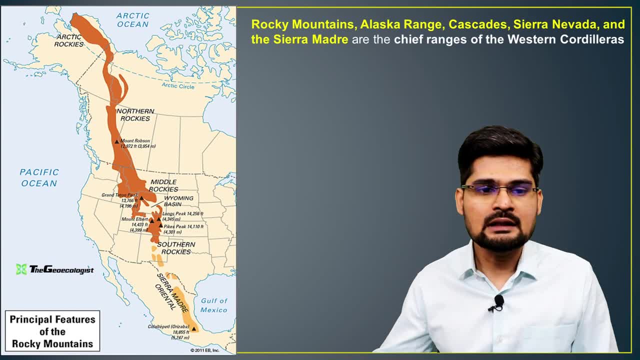 volcanism in the geomorphology lectures. now, if you go further, look into the rocky chains here: rocky mountains, alaska range, cascades, sierra nevada, sierra madri. so all these ranges, if you observe from north to south, lies in this particular belt here, right. so 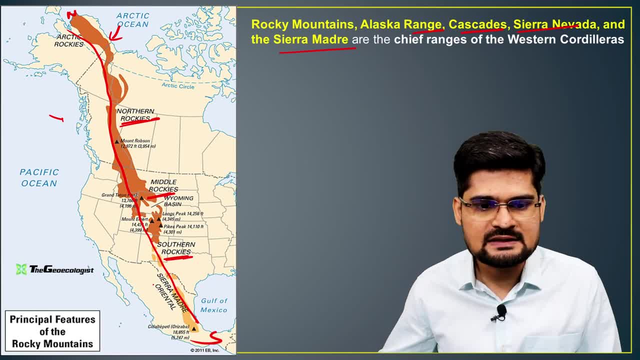 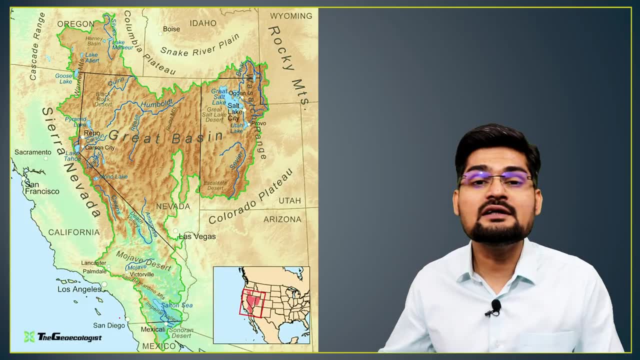 if you observe northern rockies out here, middle rockies here, southern rockies, sierra madri, oriental range here, right, so it extends from north to south. then if you observe further a very prominent feature in north america, is this feature? what is it? it's called great basin. if you observe a dry, 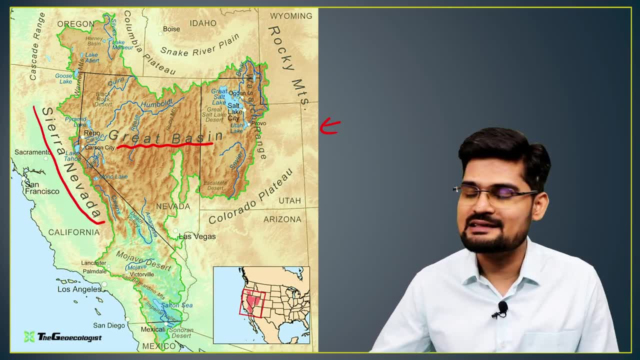 desert area in the leeward side of sierra nevada range here. it's a great basin which is a dry desertic conditions right and it is surrounded from all sides by several ranges. look here: cascade range, columbian plateau, here is a snake river plain, then you have rocky mountains out. 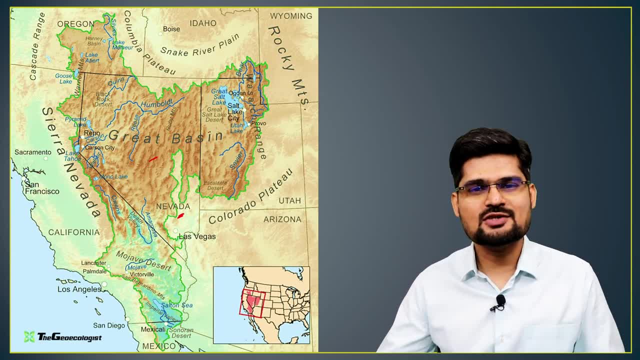 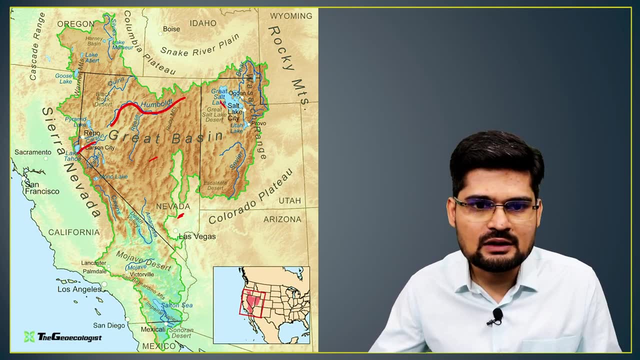 here, colorado plateau, out here now, in this great basin structure, what all you can observe is this particular river, that is humboldt river here, then you have carson city here, then you have salt lake city, in this north eastern portion of this salt lake desert, very famous, and then what you observe? 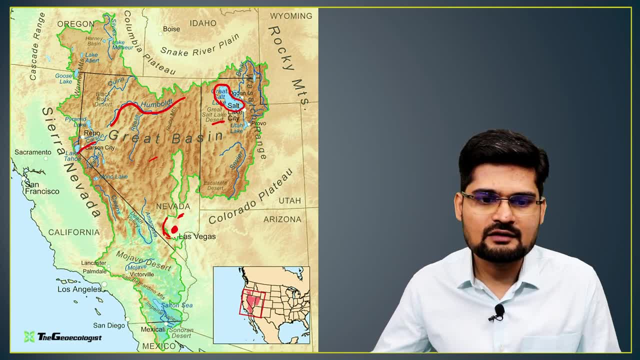 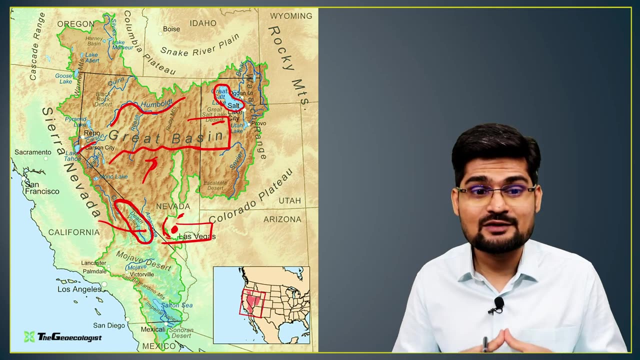 down south is las vegas, here in nevada right, a very famous city. so all these areas are there. here is death valley of california here, and this area is very famous for many touristic landscapes as well, desertic landscapes as well, and in geomorphology. we find these features very interesting, where the resemblance of 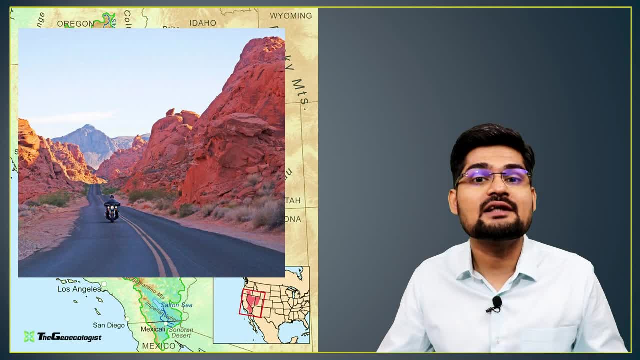 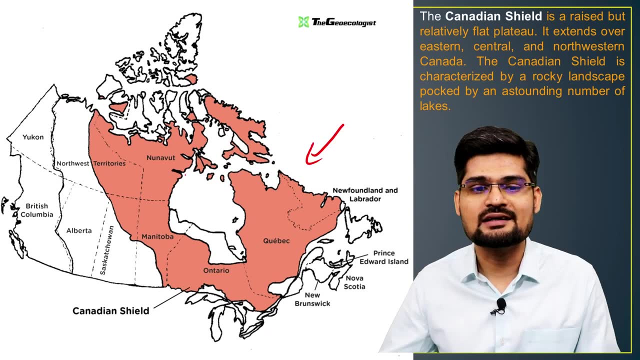 the fluvial erosion, and also the fluvial combined with aeolian erosion is found. now, if you observe further, a very prominent feature of north america is canadian shield. so canadian shield is one of the oldest systems of the world and remember, it's a flat plateau and extends over eastern, central and north western canada. so look here. 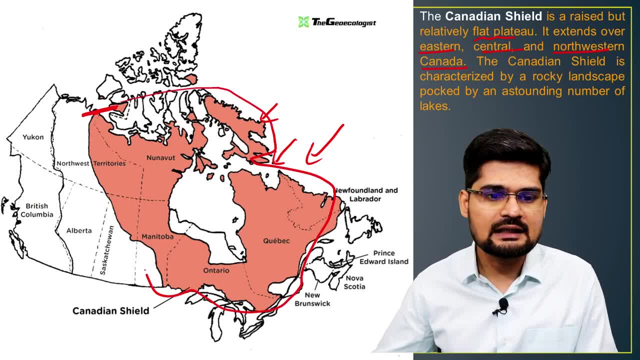 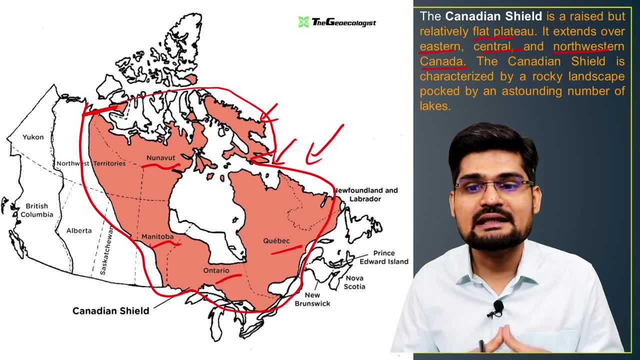 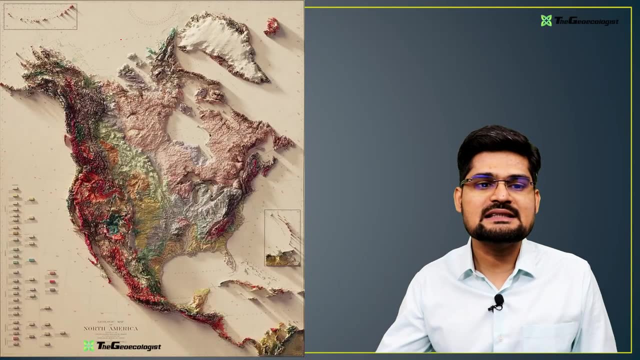 this is the extent. this entire area is part of canadian shield out here. so you have nana, manitoba, ontario and cubic as the major areas established on the shield area, and this canadian shield is majorly known for metallic minerals, if you know so, if you observe here the basic physiography. 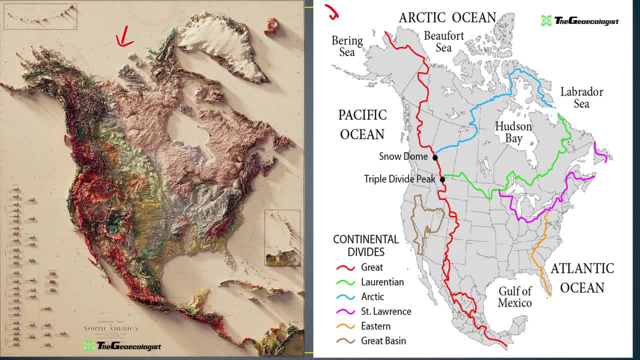 of north america. you can relate it with this particular map out here. what does it show? it shows continental divides. Look at these particular dividing lines out here. So if you observe these particular divides, these are automatically telling us the stories of how the drainage system 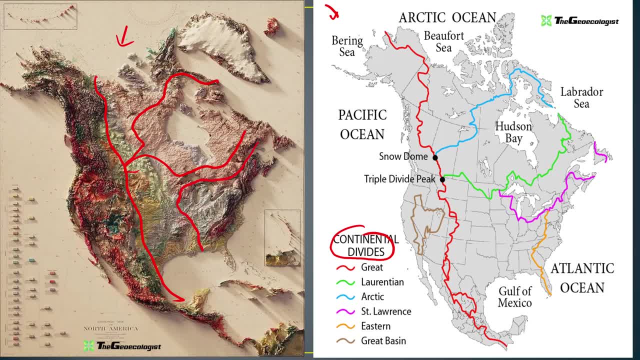 will follow or how the patterns of drainage would be demarcated or differentiated. So this is Great Divide, Laurentian Divide, Arctic Divide, St Lawrence, Eastern and Great Basin, if you observe on this particular map. But why are we talking about it? We are talking about it because it 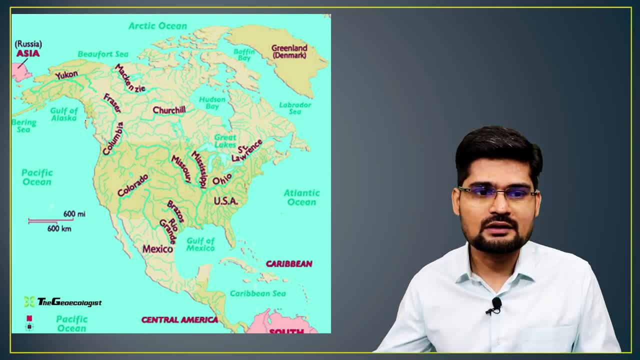 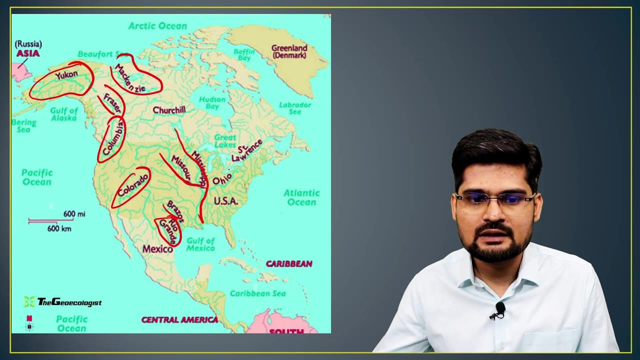 shapes the river basins of this North America. So look here, from Yukon River Basin, here in Alaska, to Mackenzie, here Fraser, out here Columbia, then you have Colorado, Bressauce, Rio Grande, and then you have Mississippi as the most prominent one here, Missouri, here, Ohio, here, and then St Lawrence. 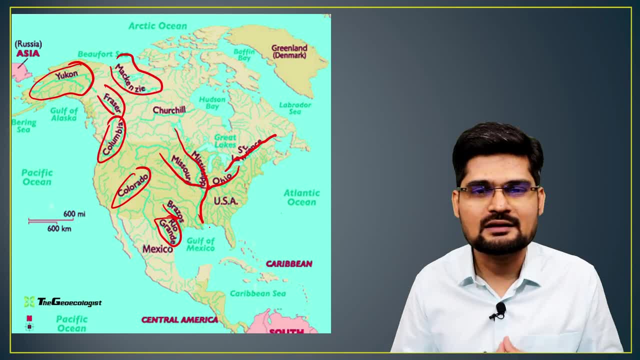 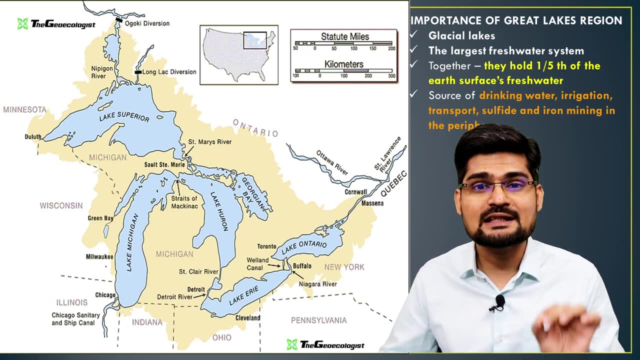 out here. These are the major rivers and there are several minor rivers in this particular continent. Now further, if you observe, is the most important and very talked about, a significant physiographic region called the Great Lakes area. Now, these Great Lakes area are coming from where? Again, remember the Pleistocene glaciation and the impact. 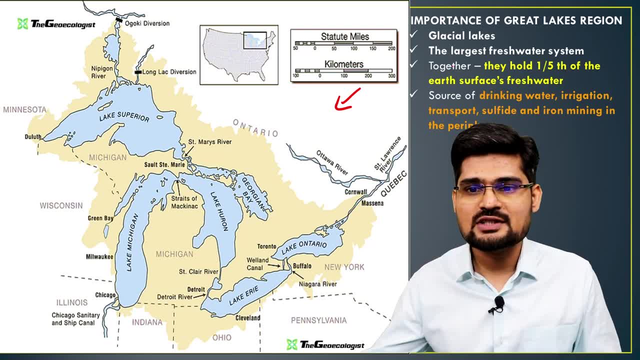 of it. So these are glacial originated lakes. So glacial origin is very important and remember: together they hold one-fifth of the earth's surface fresh water. So if you observe these fresh water lakes and the areas around it, they are the resources for North Eastern. 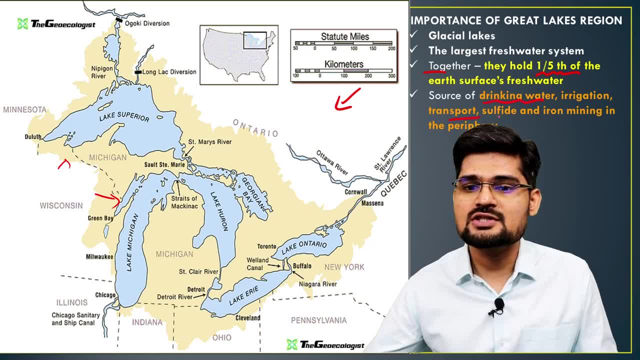 and Northern America. So observe drinking water, irrigation, transport, mining and industrial belts all alongside it. So look here Lake Superior, then you have Lake Michigan, Lake Huron, part of it is Georgian Bay. then you have here Lake Ontario, Lake Erie. So 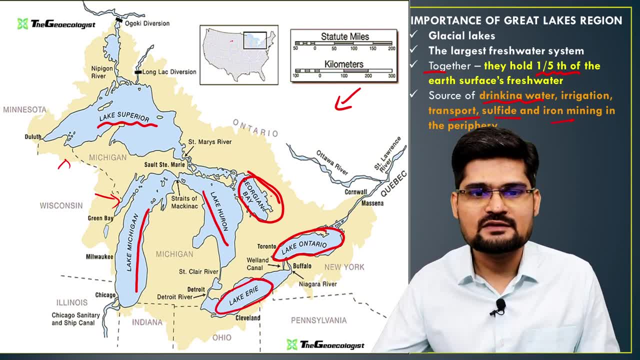 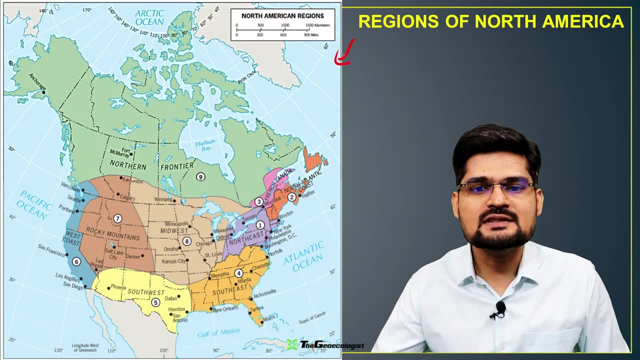 several lakes out here. these are big lakes, right? So if you observe this particular portion of America, here is this Great Lakes area. So if you observe the North American regions, if you observe through the regional lens, through aerial differentiation perspective, 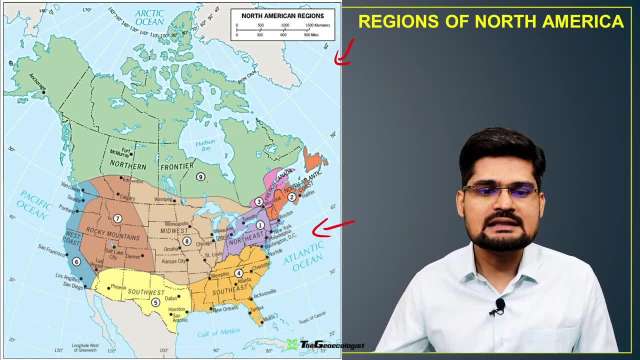 so we can divide and study the North American regions into these three areas. So if you observe the North American regions, if you observe through the regional lens, through the regional boundary of the Until the Great Lakes region, then you have these three areas. 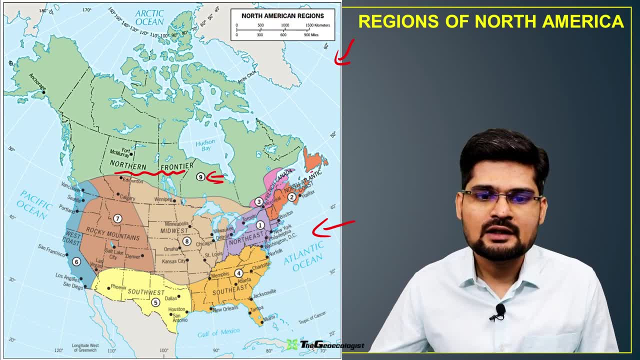 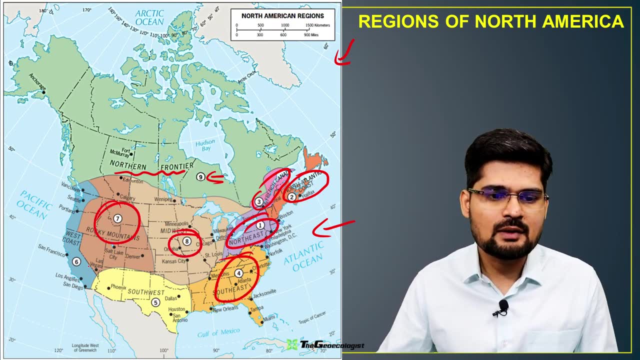 So in the North American region you have the North Atlantic coast, then you have the North Atlantic coast, Then you have the French Canada, then you have North East, then you have South East, then you have the Midwest Rocky Mountains and then you have the West. 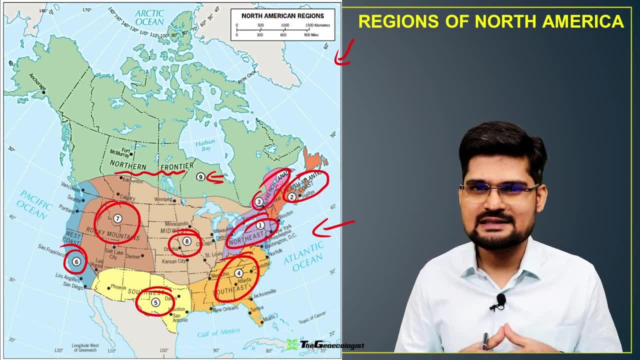 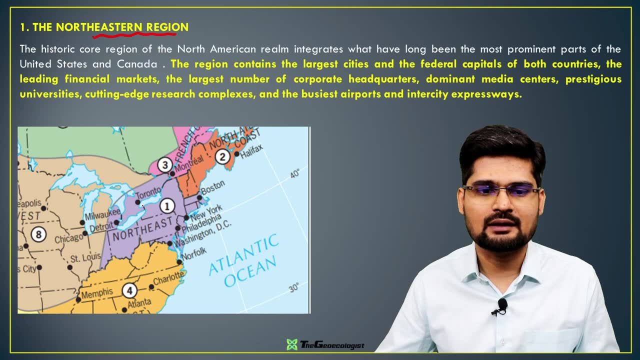 coast, then you have the Southwest. So we will be looking into each of these regions one by one. So let's begin with the first one, the North Eastern region of America, ie North America. So if you observe East, we say here: right, this particular number one. 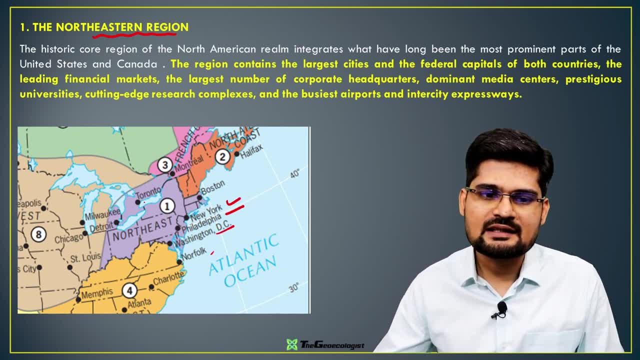 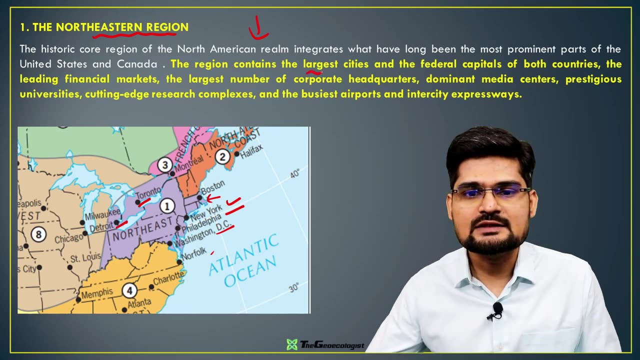 east, new york, philadelphia, washington, all these areas very famous, toronto, detroit, these are the areas which are very famous and the world cities right. so, if you observe, this is a historic realm of north america where the beginning of the colonization started. so the region contains 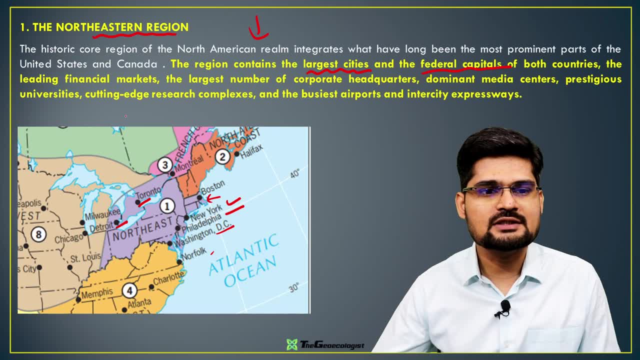 what the largest cities, federal capitals of both the countries- us and canada- headquarters, dominant media centers, prestigious universities, cutting-edge research complexes and busiest airports, international exchange centers, expressways- this is famous for the world city's creation, isn't it? then, if you observe, is the north atlantic coast that we say here. now, if you see north atlantic, 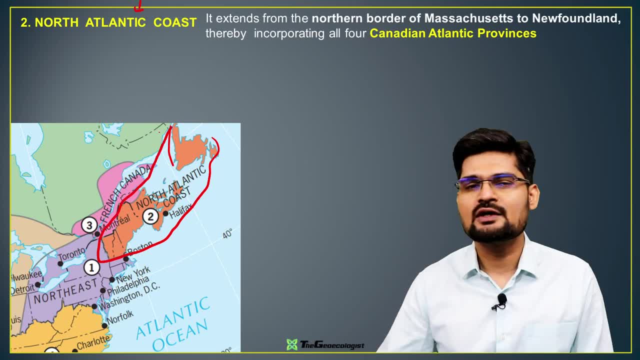 coast. this is the area we're talking about, the second region of north america, and most of it is canadian atlantic provinces, so it extends from massachusetts to newfoundland, this particular location, from boston to this newfoundland, if you observe a maritime orientation, as you can see here. 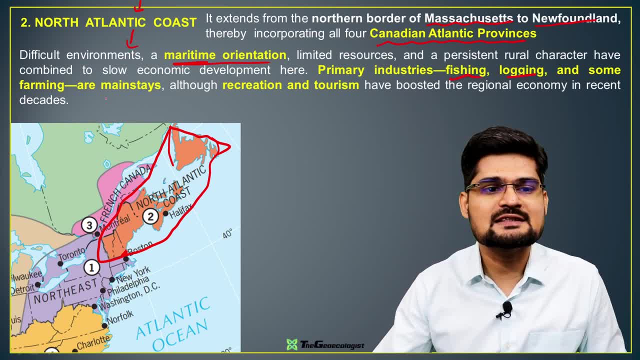 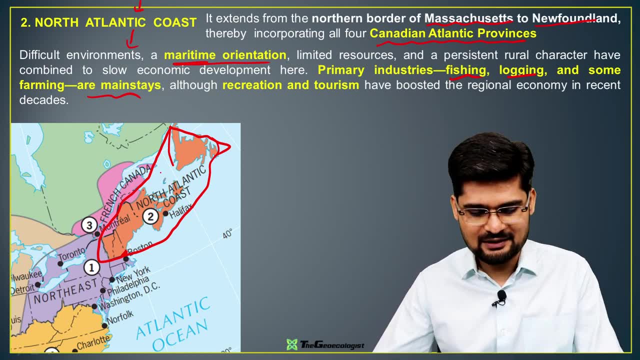 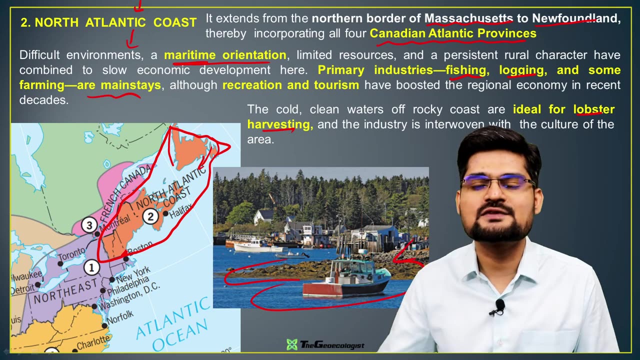 it is known for its primary industries. like philadelphia, fishing, logging and some other. farming are the mainstays, and now recreational activities. tourism is the mainstay of economy in this particular region. this rocky coast is known for lobster harvesting, so this lobster harvesting is very famous on this particular coast. now, if you observe, 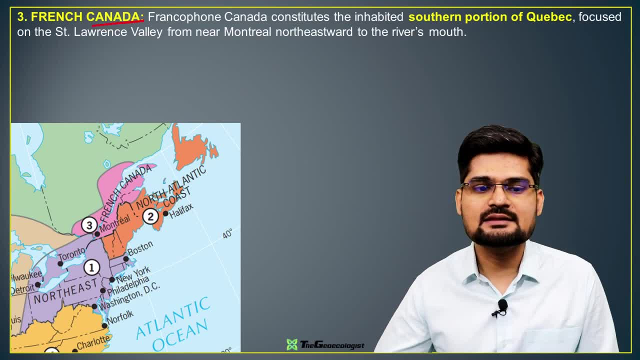 the french canada. so look here, french canada is the third one, this particular location here, french canada- as the name suggests, it was a french colony earlier- and southern portion of the cubic right. so focus on thisorders port, if you specifically for your Direction, which is over there you might face. 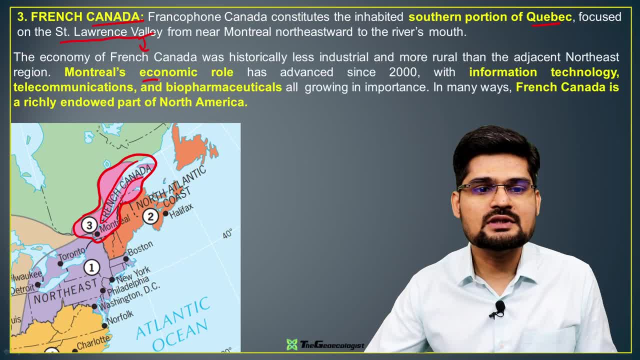 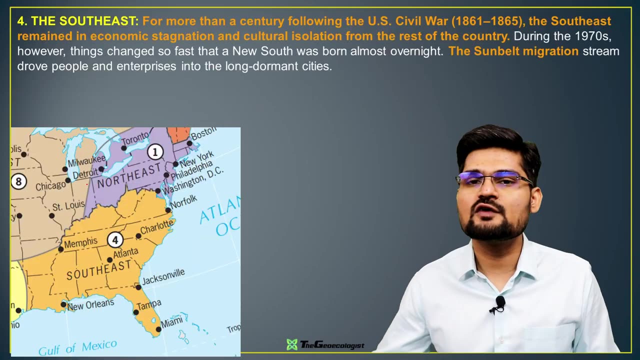 these usual mountaineers. often, though history 8 Ziploc by northern heritage, while it is the northem warner of the central sichuan cities. overall, philadelphia is the 4th and 812th arising redevelopment area, and you have here abacus & additional vision of the south eastern portion of this particular area, so that's quite a wide gap. 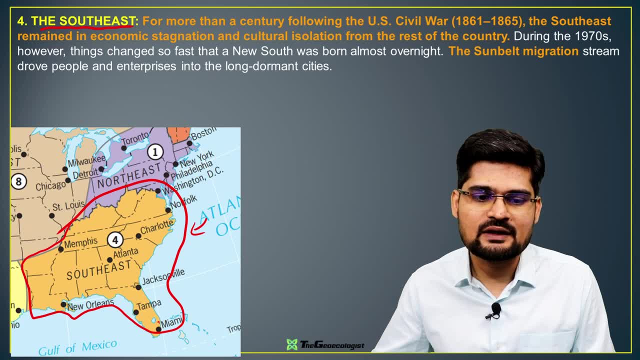 many important locations, and most important is this: florida, miami. it was tormented by the impacts of us civil war, which happened between 1861 to 1865. right, this area felt the difference because of that. then, later on in 1970s, the wave of development started many sunbelt migration. 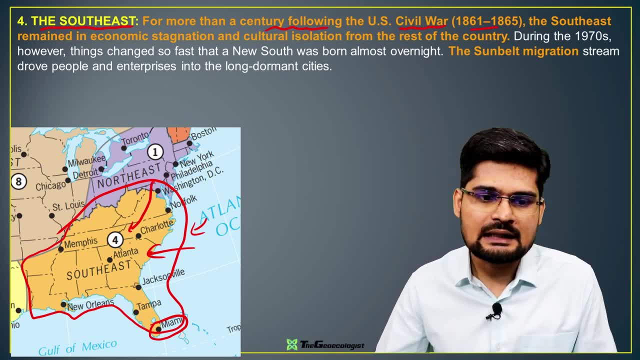 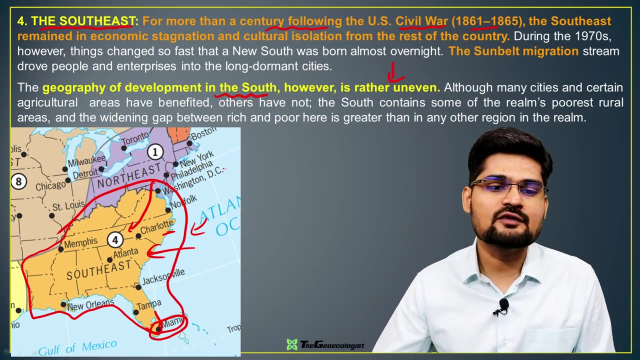 many industrial belt migration started from the north and in atlanta and other areas then in miami on this tip. so this area started to become industrialized, urbanized gradually and now it's one of the prominent areas. so geography of development in south is uneven if you compare. 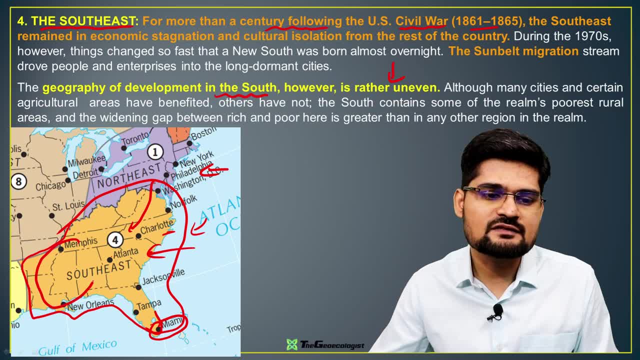 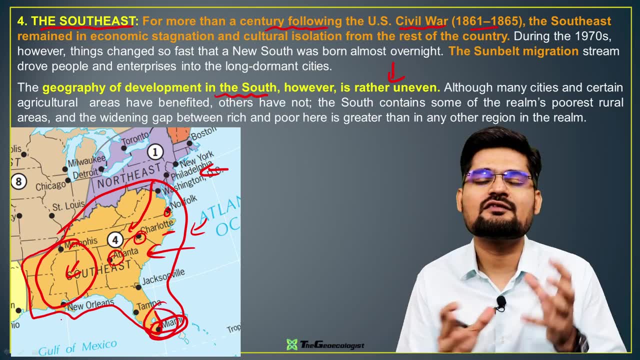 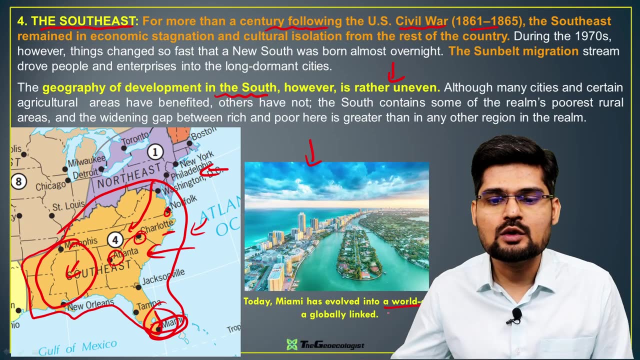 to north. so uneven development and, closely, if you observe, this particular location is not that well developed, but certain areas are well developed and so we can say there is a kind of a polarity of development in this particular realm. so, if you observe, this is miami which has become a world city. 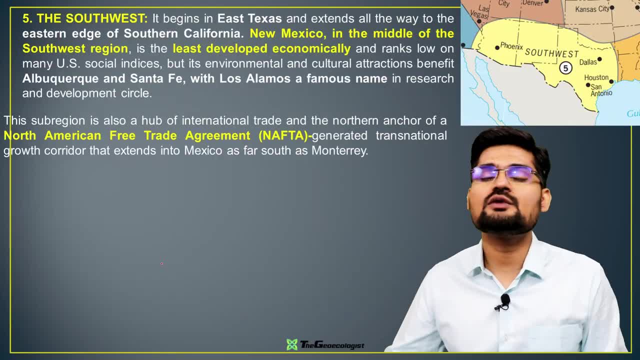 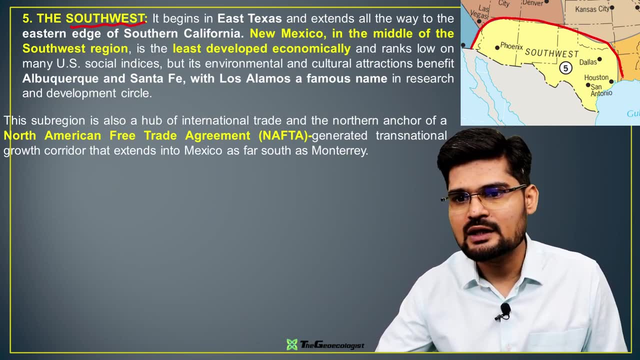 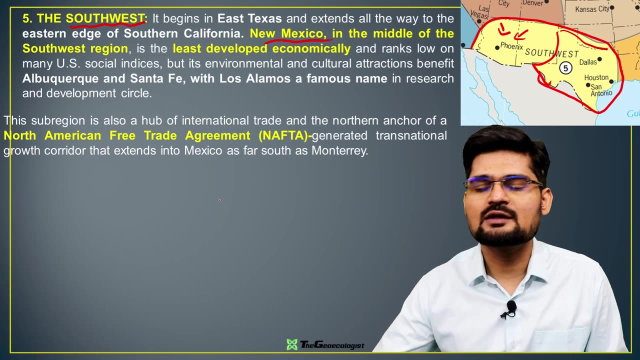 city today and is globally linked. now, if you go to the fifth one in this realm is southwestern realm of north america. so southwestern realm is this particular location. texas and new mexico are the two major areas in this particular realm and if you find that, new mexico, this particular location, 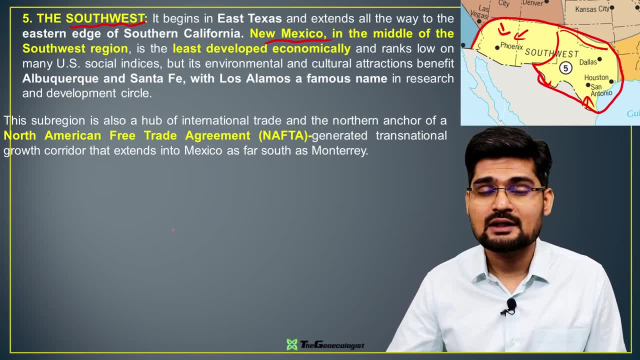 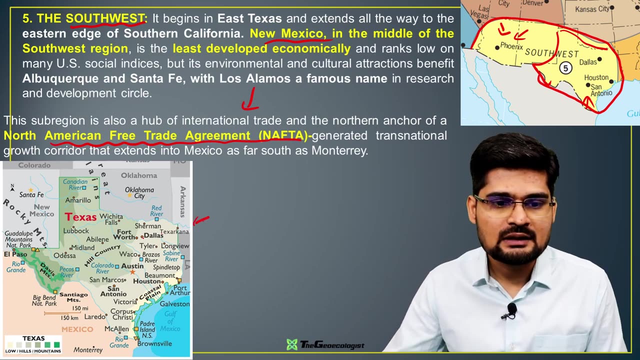 is not that well developed, while texas is the hub of economy. so, if you observe, this area is the seat of north american free trade agreement, nafta right, and it generates a transnational economy right. it's very important. and if you observe texas, this is the detailed map here: dallas, houston, this coastal 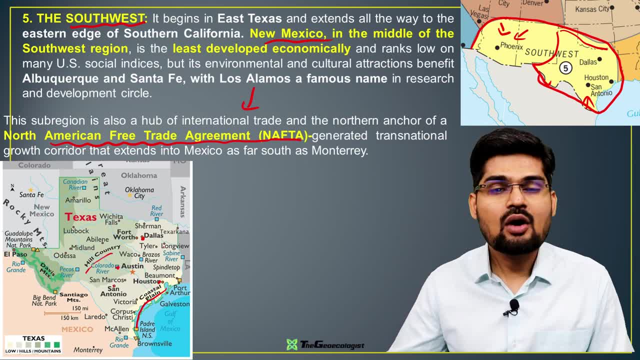 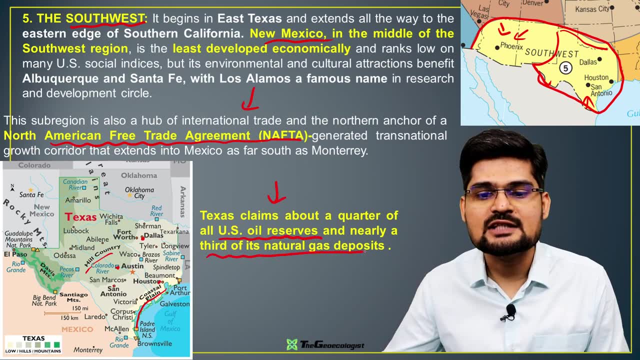 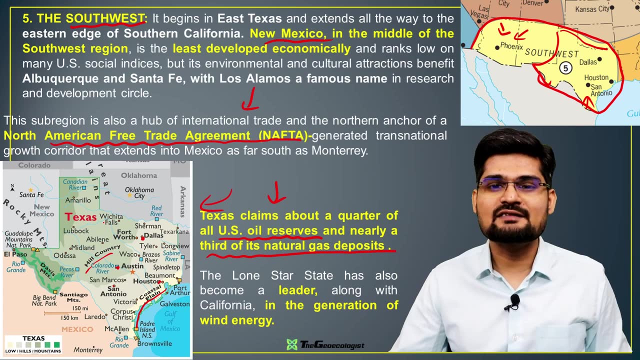 plain area, very famous, san antonio, austin. all these areas are very important and famous and texas claims a quarter of all us oil reserves, nearly third of its natural gas deposits. so that's another important, prominent thing in this particular realm, and the lone star state that we 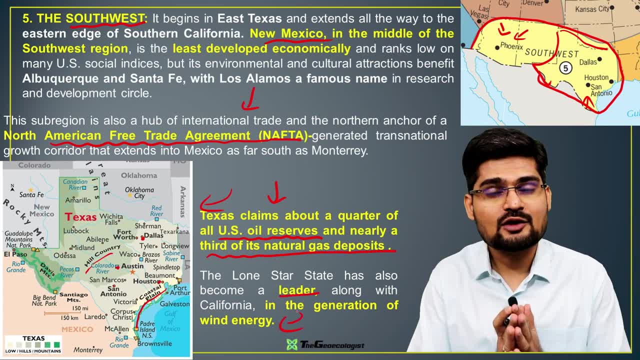 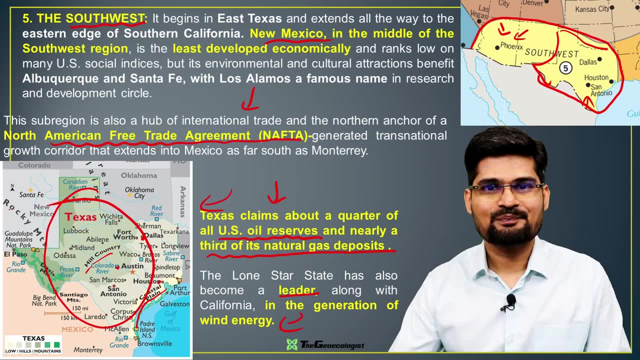 say, texas, become a leader along with california and sector of wind energy. so if you travel through this country, you'll find that a lot of windmills are there in this particular state. now let's look into the west coast. that is sixth part of the realm, so all of the california. 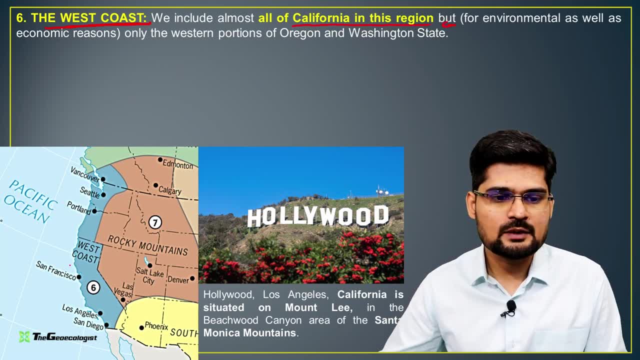 mostly fall in this region and remember this particular west coast is as important as northeast. so if you observe carefully, is the seat of famous hollywood and vancouver, seattle, portland. then you have the san francisco, los angeles and san diego. these are the major cities which are very 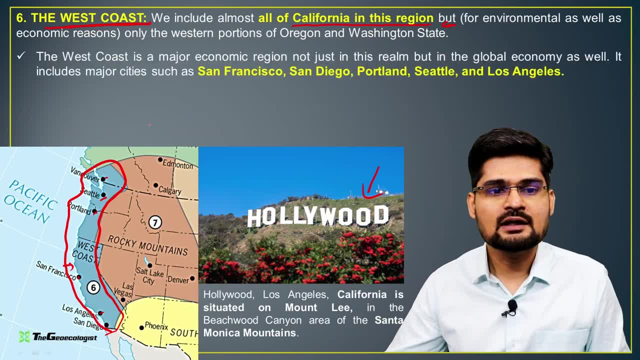 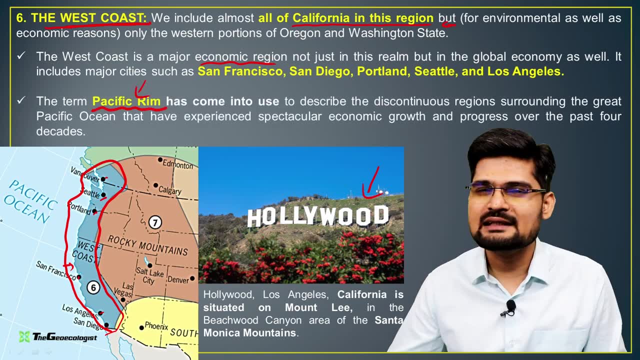 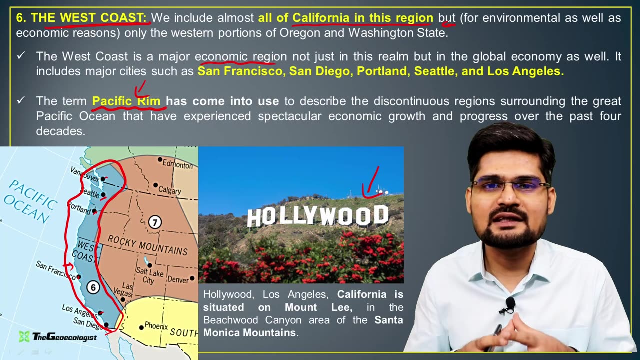 famous on this coastal area. right now, if you look further, west coast is a major economic region as we see these cities and the term pacific rim has come in recent decades to denote the developmental regime in terms of the coastal pacific areas. so these are discontinuous areas but they have high 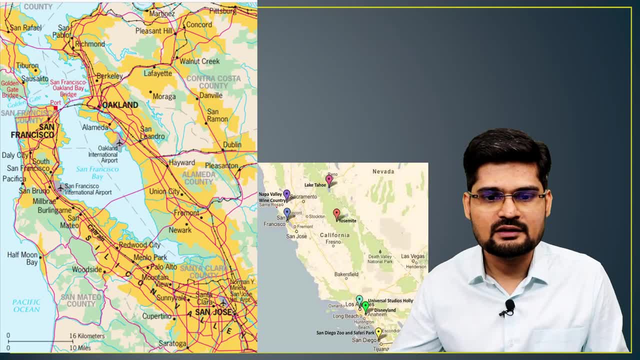 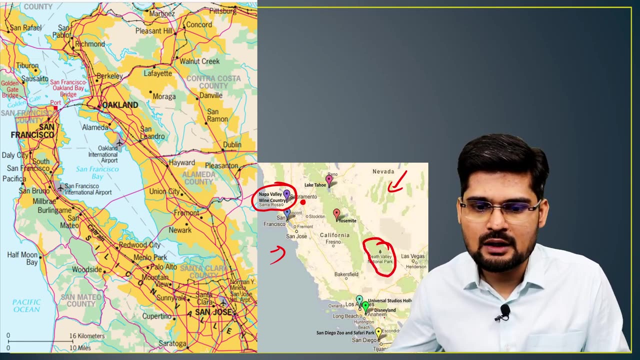 levels of development and progress. now, if you observe carefully here, this particular location here. so look at these particular places in the california, very famous, so this is the capital. then you have napa valley, famous for wine, then you have these areas like death valley national park, then you have disneyland, universal studios, hollywood right, los angeles, then you have long. 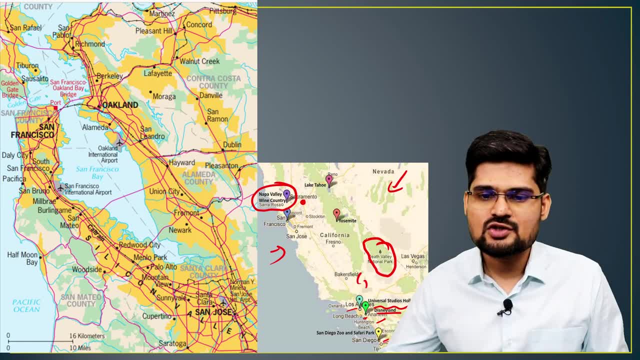 beach, huntington beach, then you have san diego and adjoining nevada, where las vegas is there. so this area is very famous for physical portion, physical geography, in terms of yosemite and other areas which have very prominent geological features and also human features, if you observe. 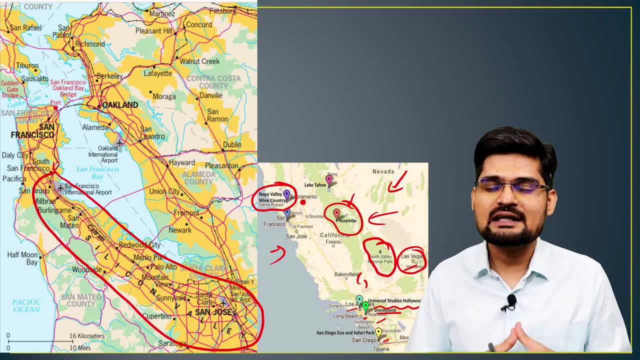 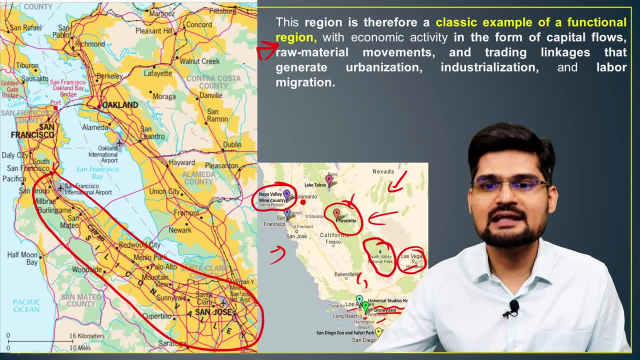 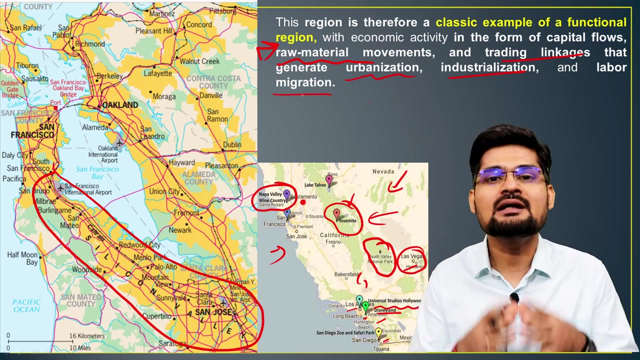 films here to düa del rio, MeinungII, whatever use, whether you are a tourist traveling, and also here is the second location, which is theğin. here you can see something very numerous assistant now further the rocky mountains region of north america. so you observe this. 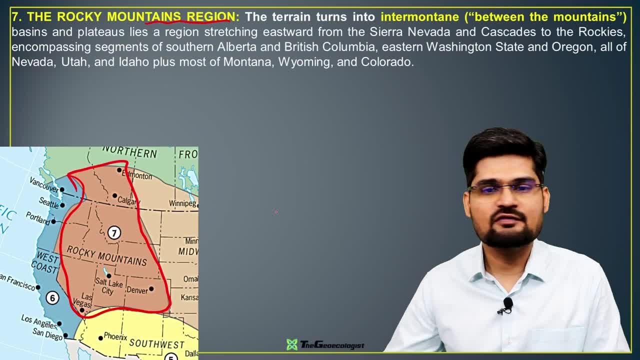 rocky mountain region here, this particular region, which is famous for rocky mountains and it's an intermountain plateau that we say between the mountains. this area has the southern alberta, british columbia, eastern washington state, oregon, then you have nevada, utah and idaho. so if you 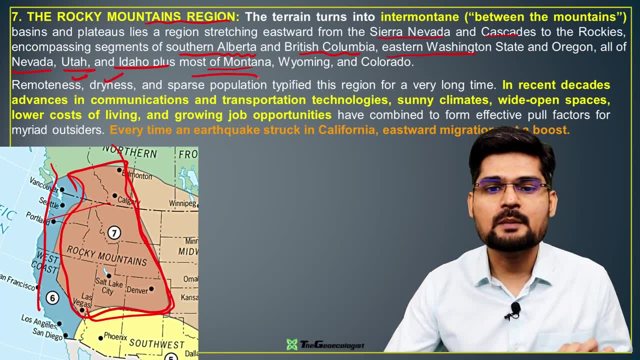 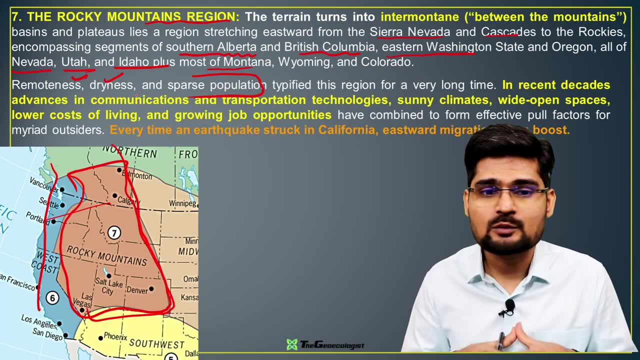 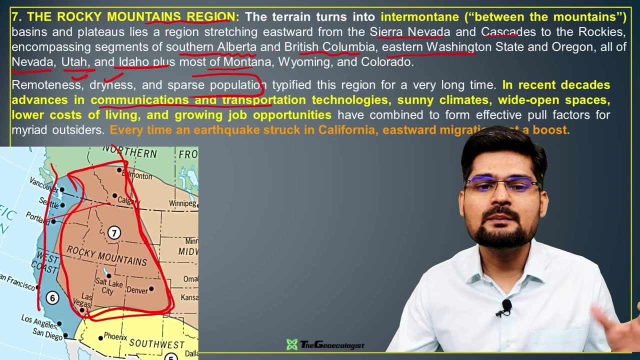 observe the remoteness, dryness and sparse population is something which is very important to note in these areas, then the question is: why is this area famous? are people not moving into this? remember, in recent decades, with advancement of communication and technology, transportation, housing, now people are moving into these drier areas as well, and now, every time an earthquake. 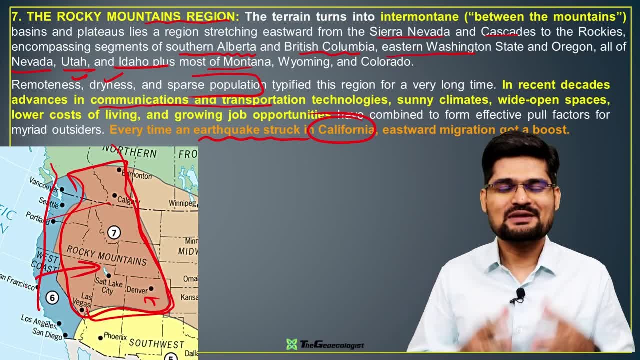 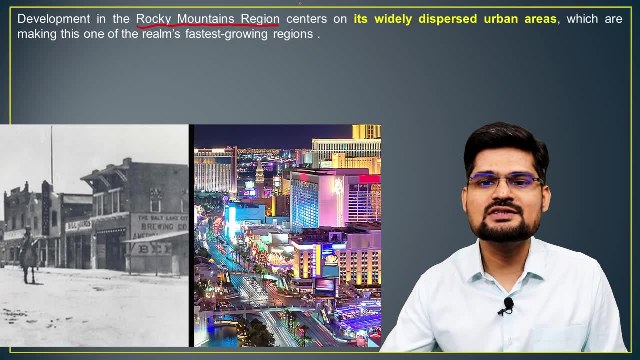 struck in california, people tend to move eastward. so there is a very interesting reason for people moving eastward gradually with development. then, if you observe the development of rocky mountains region, where the centers opened up gradually, one of the famous areas is that, you see, is las vegas. 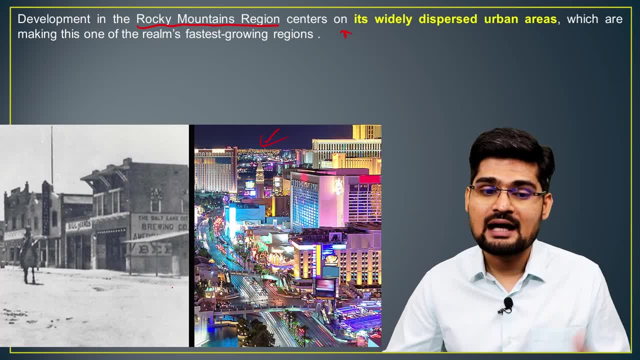 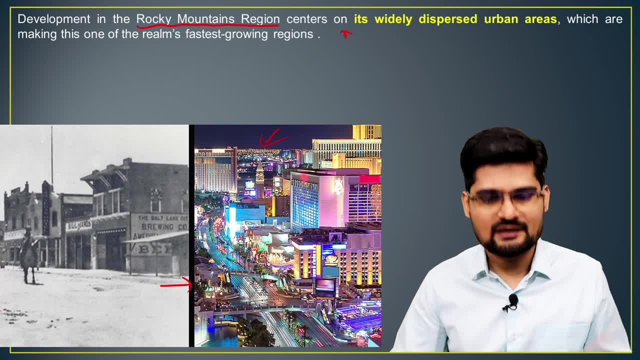 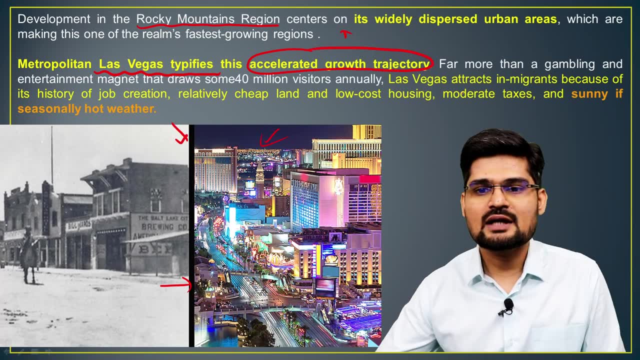 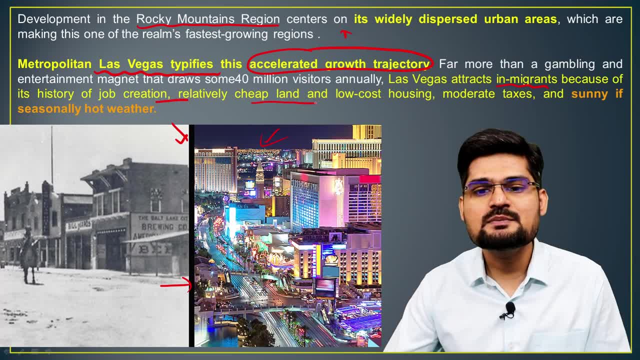 immigrants from other areas because of job creation, cheaper land, low-cost housing in its vicinity and also the famously casinos which are there, for which it is known in the world tourism industry. then the midwest us. this is where vast north america- heartland you can say- is there and remember chicago, which is one of the major cities in the world, which is known as the world tourism industry, then the midwest us- this is where vast north america heartland you can say is there. and remember chicago, which is one of the major cities in the world tourism industry, then the midwest us- this. 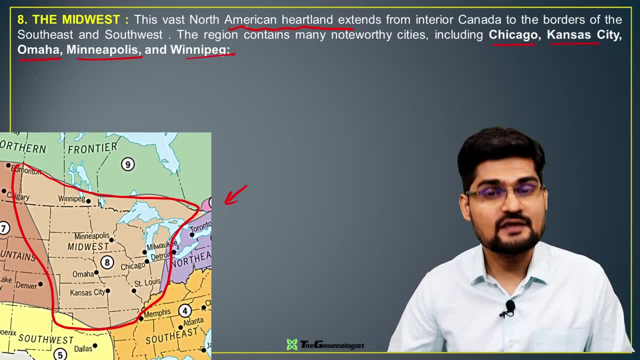 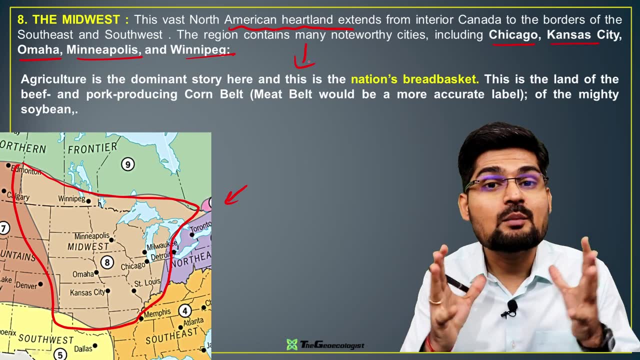 is where vast north america heartland you can say is there. and remember chicago, which is one of the major cities in the world, tourism entity c, expensive, densely populated reality fitch sign. simplify: how much money does langiston UC tolerated? all these areas are very important for United States, so agriculture is the dominant glory here and this region is called nations bread. 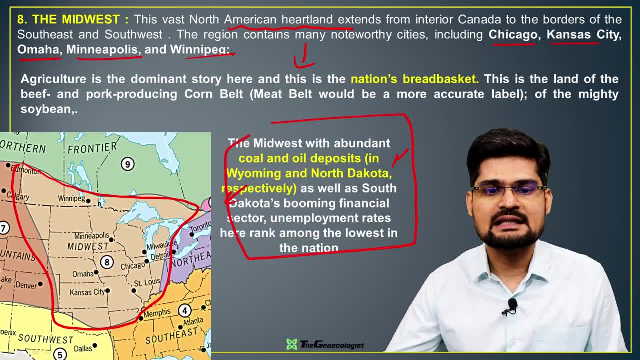 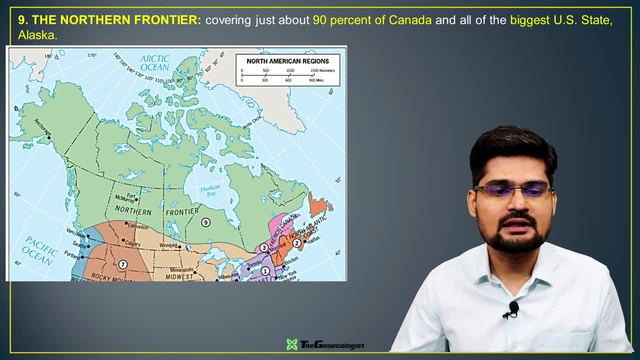 basket and the Midwest, with abundant coal and oil deposits in Wyoming and North Dakota as very important here. now let's look into the 9th and the last Frontier, which is the northern frontier part of the North American realm. so ninth region, if you divided ninety percent of Canada is thee and the last is the northern Frontier, which is the north American. 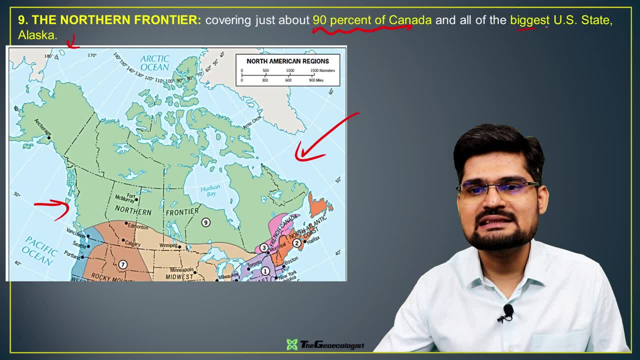 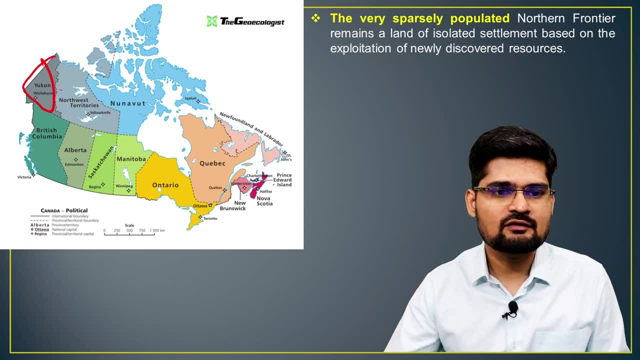 is 90 percent of canada and alongside the biggest us state, alaska, it is there in the northern territory. so if you observe the canadian portion, this is yukon, then you have northwest territories, here, nunavut, here, then you have british columbia, alberta, then you have manitoba, ontario, quebec and 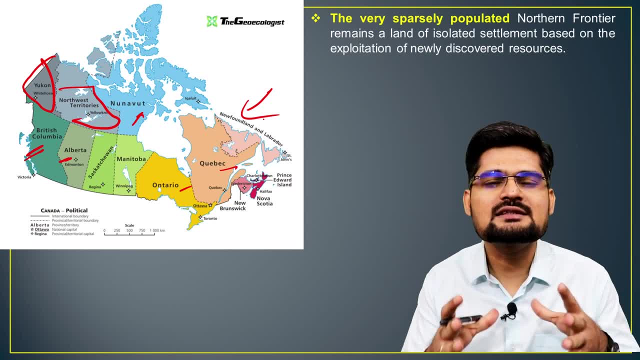 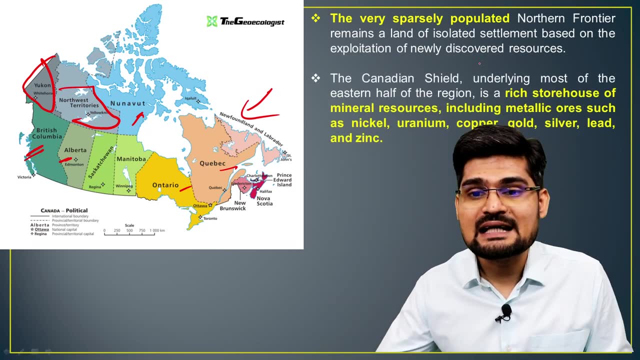 several others. this is the location and it is a very sparsely populated area of the world, as it is known. but it's not famous for population. rather, it's famous for the minerals that it has. it's a rich storehouse of minerals. remember mineral resources like nickel, uranium, copper, gold, silver. 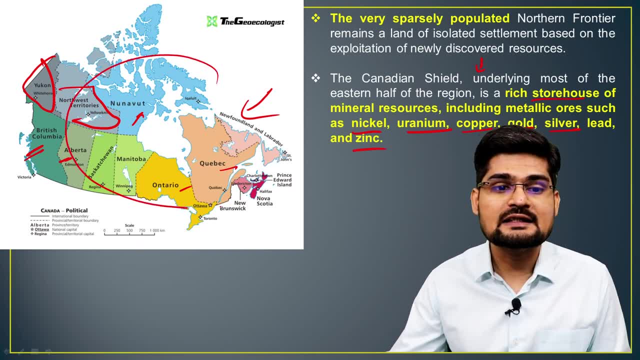 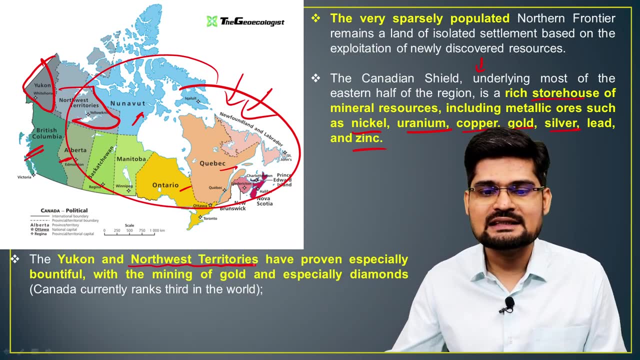 lead, zinc. all these are found prominently in this particular region and it's the seat of canadian shield, as we learned in geology. so, if you observe, the yukon and northwestern territories have proven spatially bountiful for mining of gold, so this is where gold mining is done right. and if you observe, 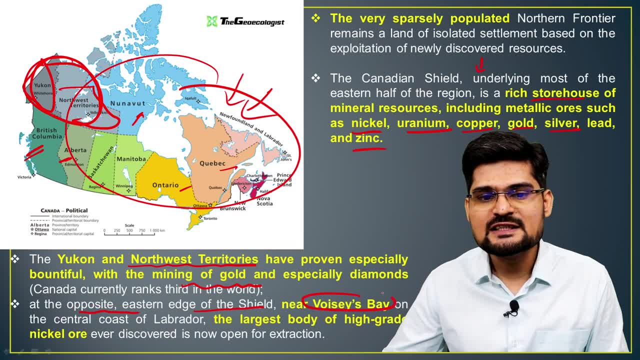 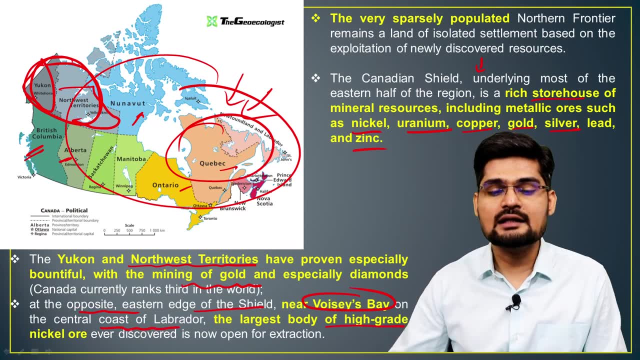 at the opposite eastern edge of the shield, near vosis bay. if you observe, this is where gold mining is done- right. and if you observe at the opposite eastern edge of the this particular location, right. this is famous for the high grade nickel ore and other extractions. 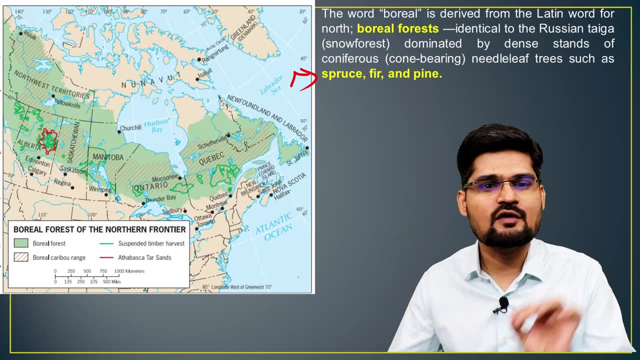 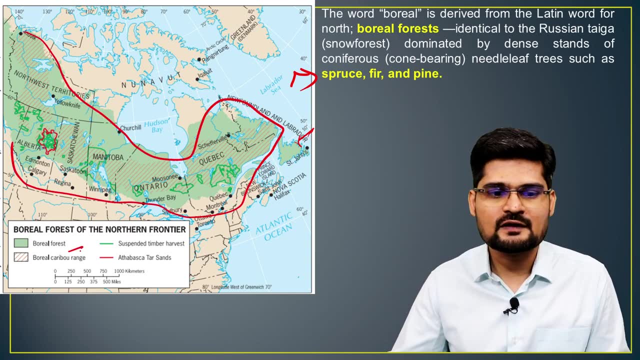 that are done. and one more important point here is the boreal forests, famous in canada, which is found here. so this entire green region, if you observe, is famous for these boreal forests, and not just boreal forests but some wildlife species as well. so if you observe here the wildlife species, 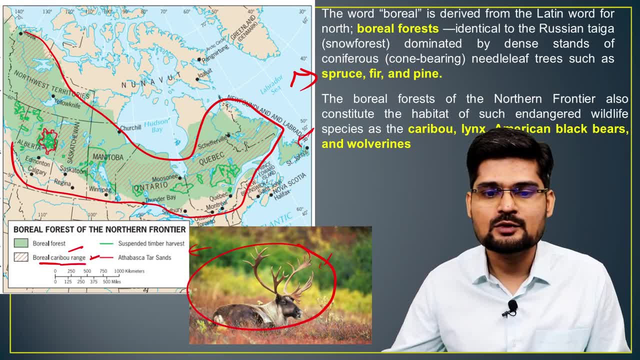 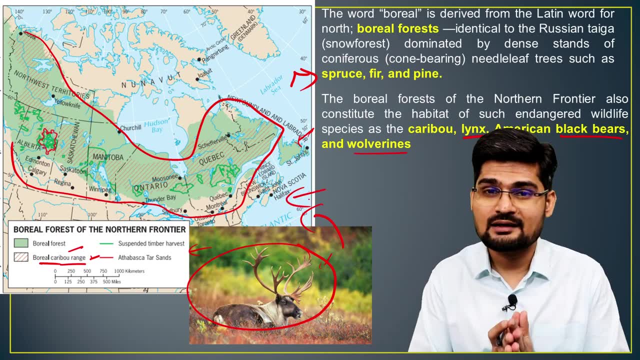 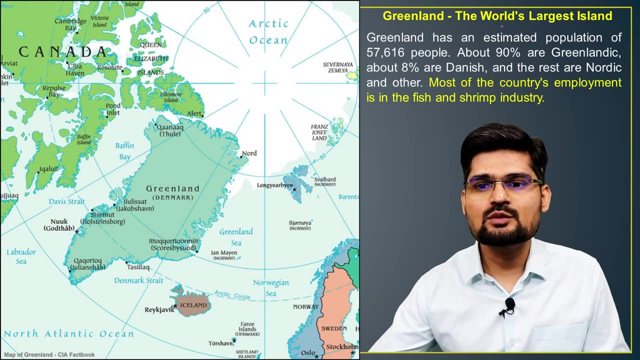 the boreal caribou range. this is boreal caribou, which is endangered species. other than that, lynx and black bears and wolverines are also found in this particular area, so it's important for biodiversity as well. now let's go into the greenland area, the island. so greenland is the 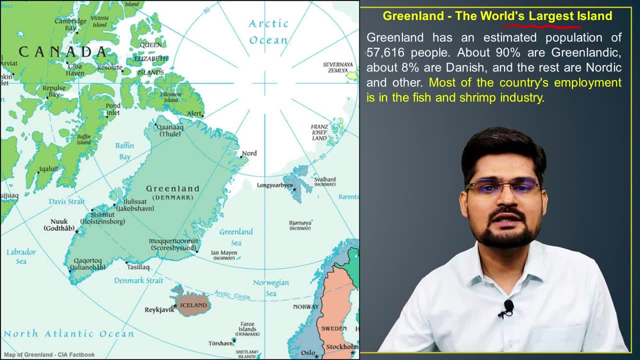 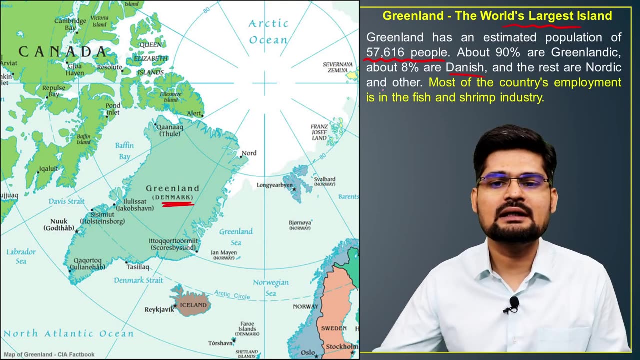 world's largest island, if you observe in terms of islands and remember it's very sparsely populated: 57 000 around population, 90 percent are greenlandic and 8 percent are danish. now this is part of denmark, right as in administration it is part of denmark and most of the country's employment is. 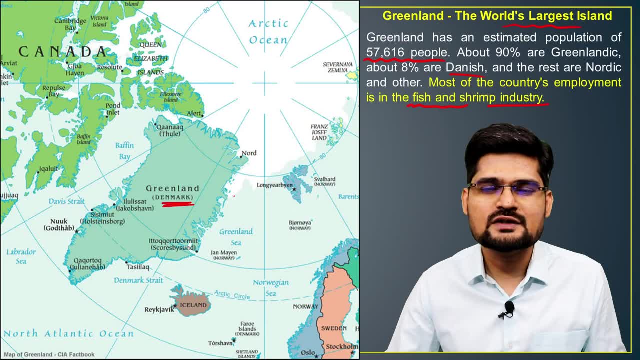 either coming from fishing or from agriculture. so this is part of denmark, and most of the country's employment is either coming from fishing or from agriculture. so this is part of denmark, and most of the country's employment is either coming from fishing industry, shrimp industry or little of tourism. 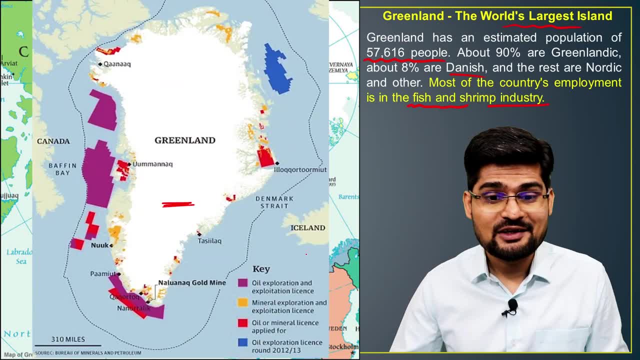 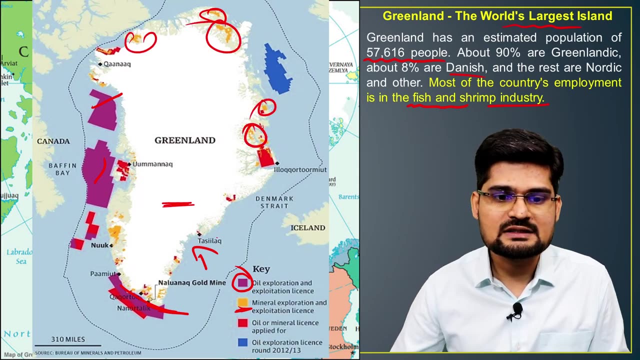 but now it's famous for some other reasons as well. if you observe the new age mining and oil exploration. so look at these areas, these purple belts, these are all oil belts. here then mineral belts, if you observe, are these particular mineral belts spread across the coasts of green land and 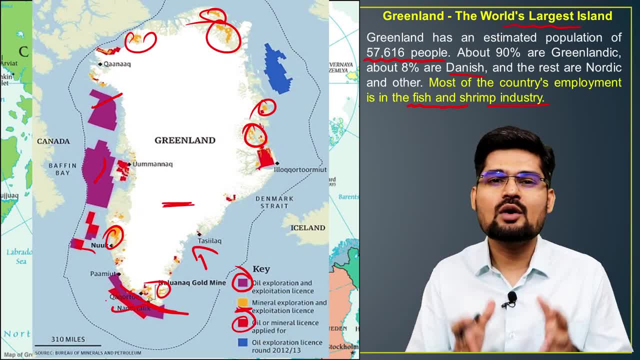 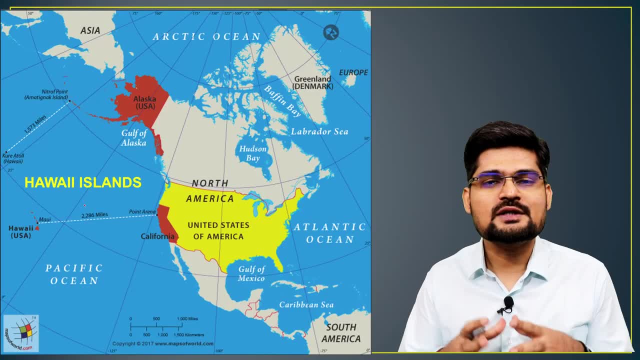 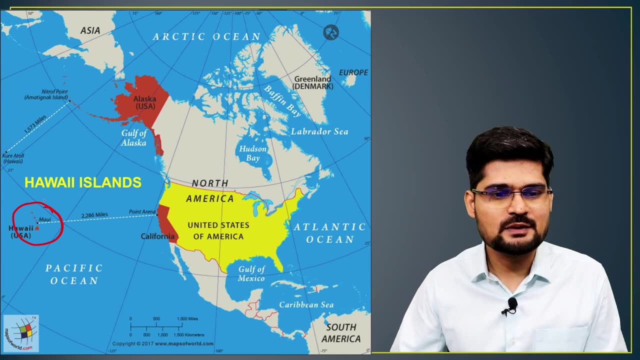 oil exploration is all red areas. so minerals, oils, metals- these are the things which are now bringing people to greenland. now, if you observe, one of the most important areas in terms of the north american islands is the hawaii island, the chain of hawaii island, the archipelago and nearest 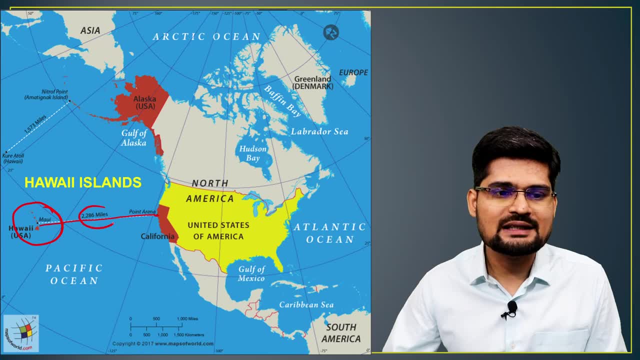 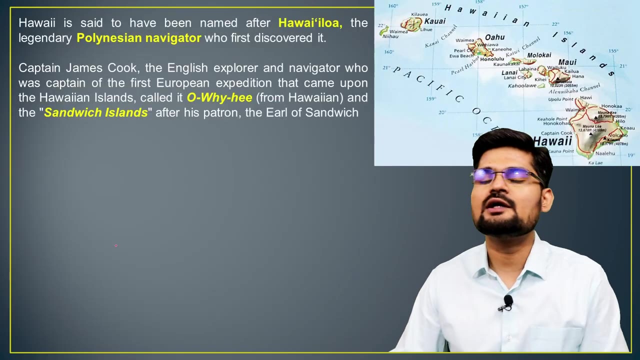 point, if you observe, is here in california, two to eight, six mile apart from this curie atoll of hawaii. if you see here distance from alaska, this particular point is nearest. so this is the location and, if you observe, it's just crossing around tropic of cancer here. so let's look into the hawaii. 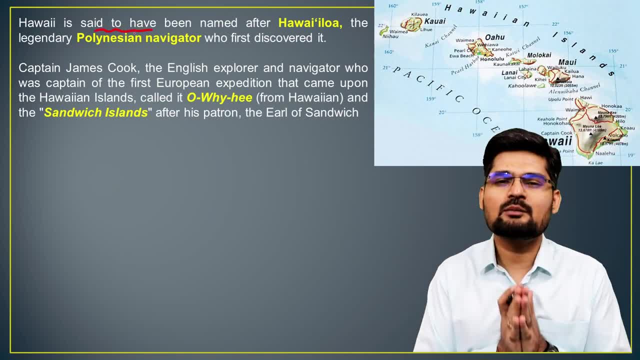 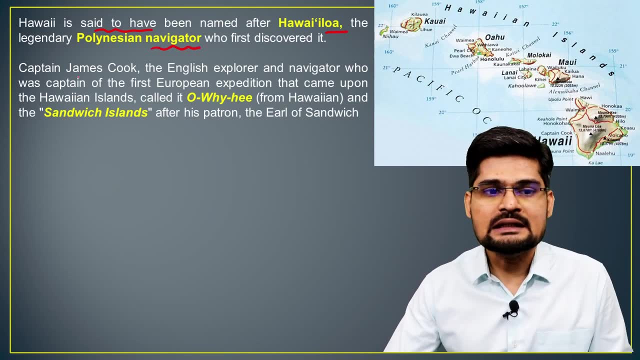 and chains. so, if you observe, hawaii is said to be have named after hawaii loa. this person was a polynesian navigator who first discovered it and later, when james cook, an english explorer, and he named it- oh why- he from hawaiian and later also called it sandwich islands because of his patron. 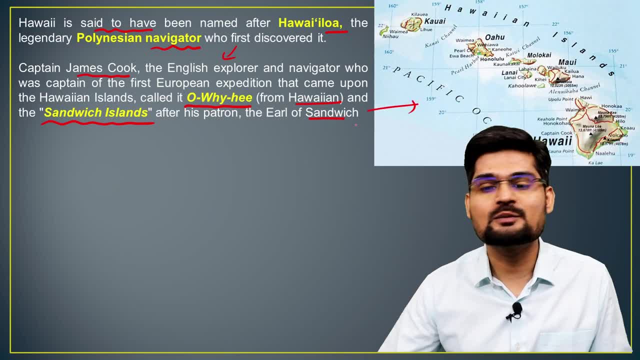 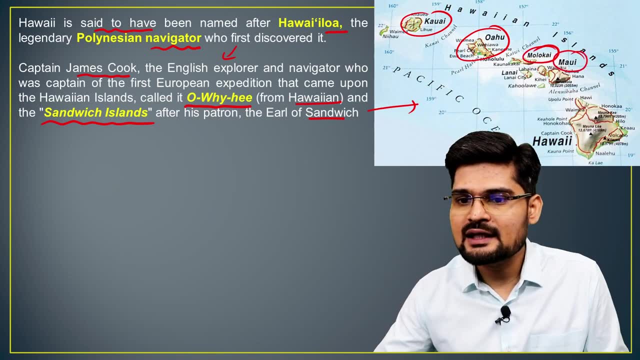 his sponsor, earl of sandwich, so that's why it's also known by the name sandwich island. so look, here you have kawaii, then you have ohau, then you have molokai, then you have maui, then you have the biggest one, that is, hawaii. and if you observe, honolulu is here on ohau and pearl.